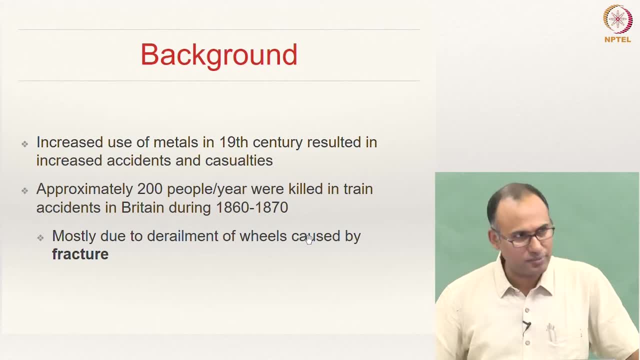 or the birth of fracture mechanics, or the need for fracture mechanics primarily arise after industrial revolution, When people started using the metals in a large quantities and you see machine components or structure made of these materials every, almost all walks of life, and particularly with the increased use of these metals around 19th century, people have observed increased 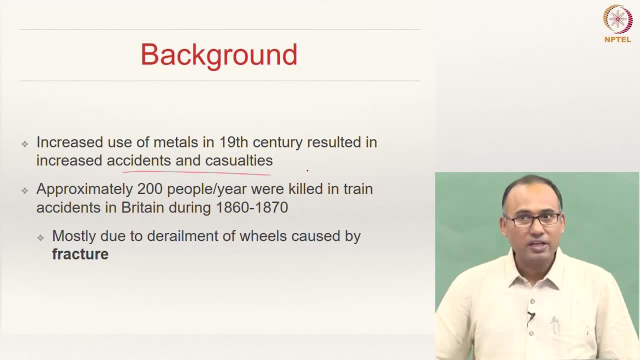 number of accidents and casualties. In UK alone, there are approximately 3,000 accidents per week. So in UK alone, approximately 200 people per year were killed on worst brick works. Oh, This is something which doesn't. this is also taken from the Loki Sooakti movie. 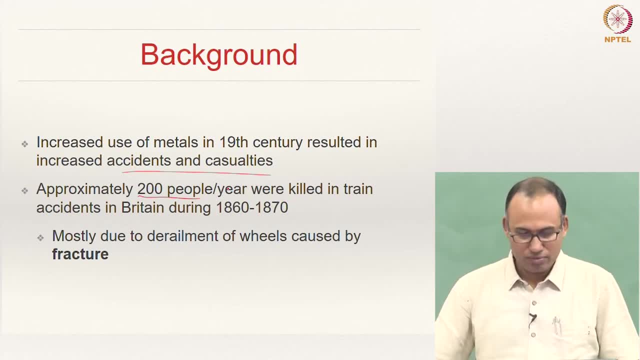 There are approximately 200 people per year who are killed for train accidents alone. So the early railway was there in UK and also in mainland Europe. So in UK alone they have observed, they have had reported 200 accidents per year, particularly around 1880s, so on, And most of these failures or due to 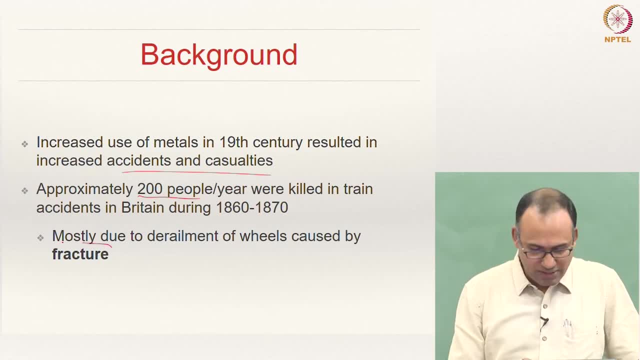 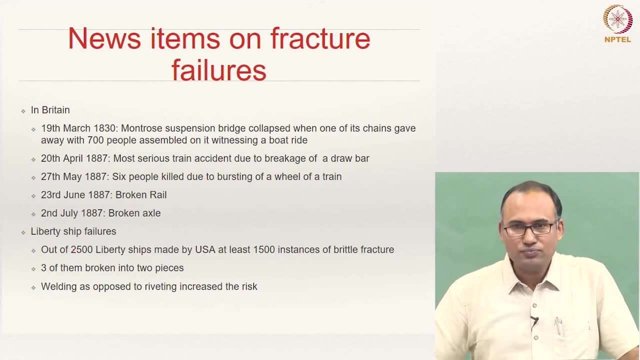 or axles and so on. So the main reason for them was the fraction. So there are certain news items around that time in Britain. So in 1830, a suspension bridge in Montrose collapsed when one of its chains gave away. They broke and about 700 people- while there are about 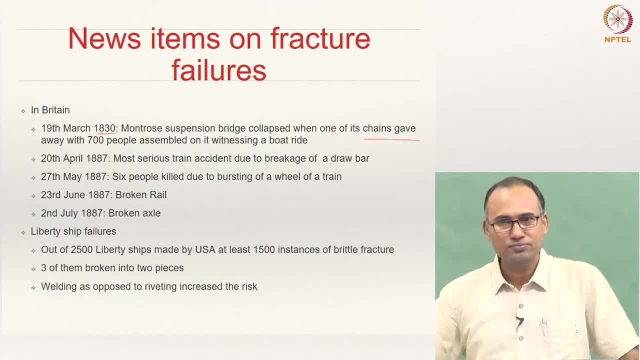 700 people standing on it and watching a boat ride. one of the chains broke And in 1887, this is the time this year- it seems to be a dangerous year as far as train travel was concerned. On 20th April they had most serious train accident due to breakage of a drawbar. 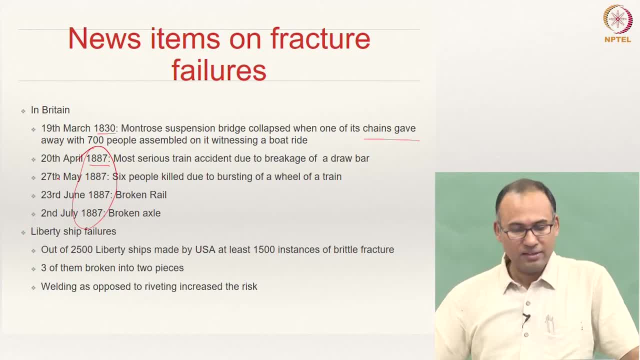 in the right in the train And then one month later they had a major accident. One of the wheels got burst off. That means there was a crack, and then the wheel gave in. Another month later there was a rail that was broken. A month later there was. 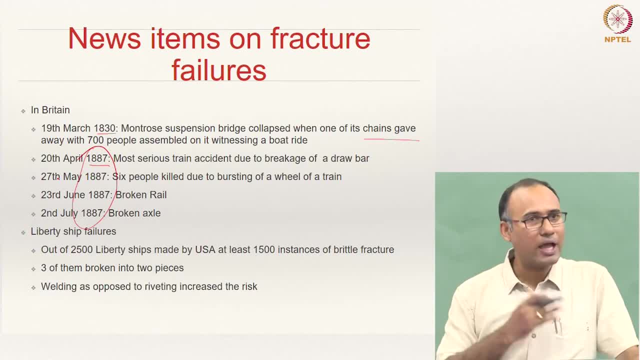 an axle that was broken. So these accidents were happening very frequently. Every month one accident, you can imagine, right Today. it is obviously not possible to ask people to travel by train if you have something like that right. So there are not only train accidents, there are also other kind of accidents. This is 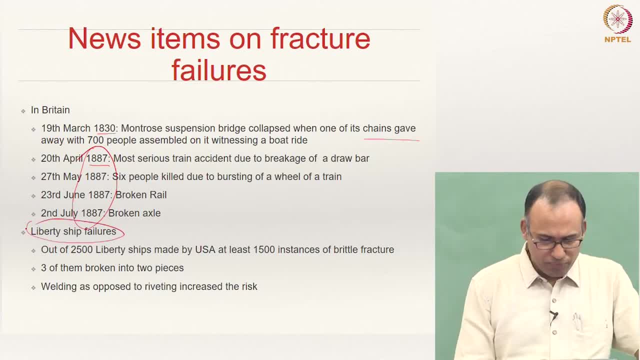 during World War. the Liberty Ship failure is one of the very saddening stories, but it is actually one of the most critical problems that actually led to the study of fracture mechanics or fractured bodies in detail. So the Liberty Ships: The original design was in UK, but then USA had to make these ships in large quantities. 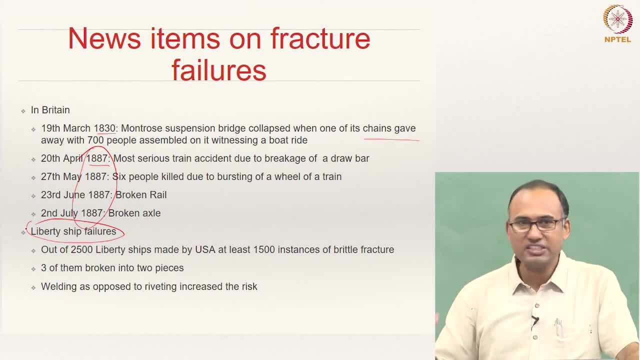 but in within a very short period And the original design had riveted joints. But if you have to do the riveted joints of your hull ship structure hull structure it takes longer time. So the design, the designers or engineers in that railway was a bit short. That is why we have to do some. 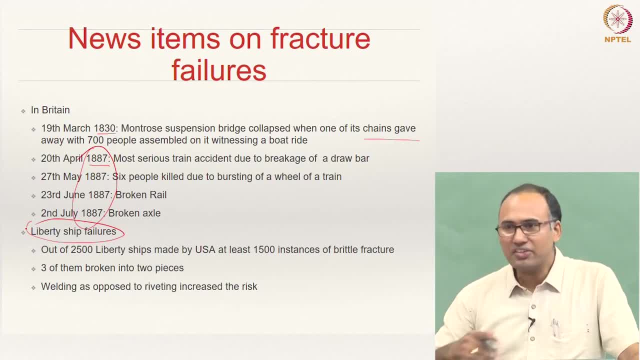 ref Piece Re핑, and that is the important thing, but it was more of an task towie about. the United States thought, okay, because it takes longer time and we do not have enough time. they took a call saying that we will do a welding joint rather than a riveted joint. 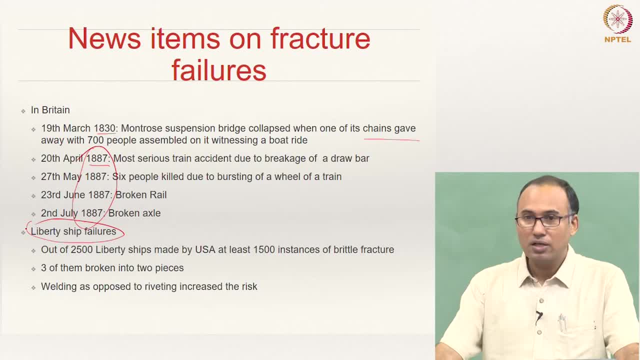 So there are about 2500 ships were made, of which just by this small design change, actually a small manufacturing process change from riveting to welding, There were about in operation. there were about 1500 instances of brittle fracture And most severe of them is three of them actually broke into two pieces, like it is not titanic. 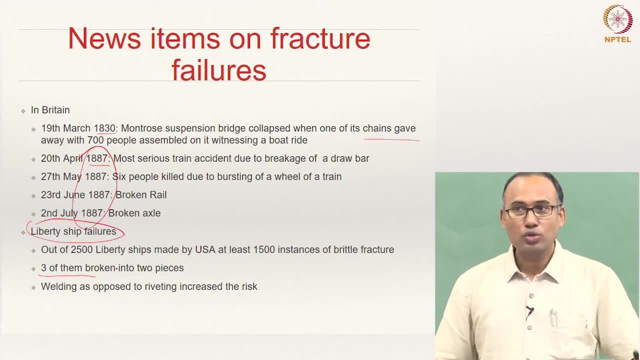 okay, these are all warships. So two of them actually broke into two pieces And later people started to say that this is not titanic, this is not a ship, this is not a ship. And later people found out the reason was the welding process that was adopted as opposed. 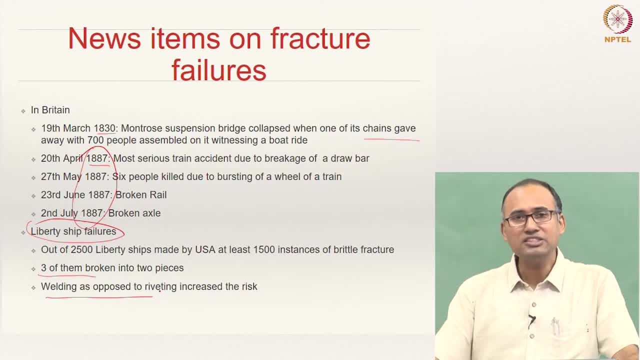 to riveting process and it is not really completely welding process, because when you have welding you are prone to have these micro cracks and they may grow in size and then you may have pores. So there are possibilities for you to have initial imperfections like air holes and so 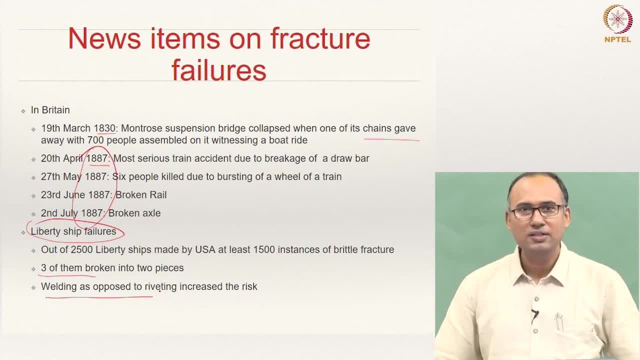 on They might actually grow in size to a large crack and then eventually they may break right. But there were also other reasons why it actually broke. it is not only that people really did not thought about something called ductile brittle transition, A material which is ductile at room temperature. when you reduce the temperature of the material, 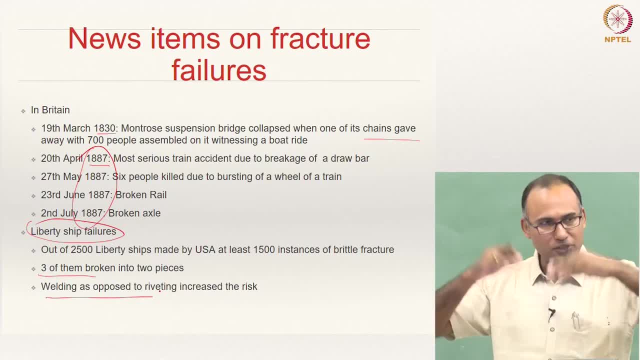 it actually becomes brittle at very low temperature, And that is something that people did not clearly pay attention to, because these ships were sailing in during the World War. they have to sail to Europe, right, they are fighting for, And in Atlantic the temperatures during winter can drop down significantly. right, and they 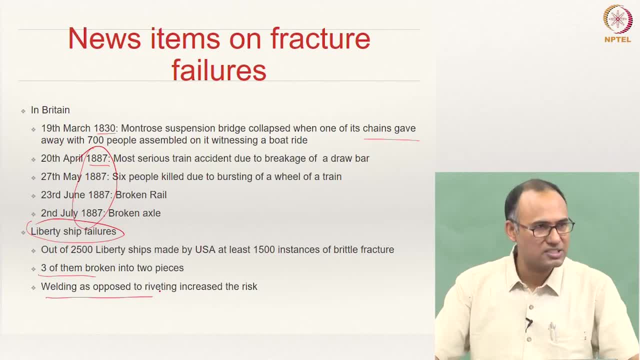 did not really think about these. ductile, brittle- Okay, Okay, Thank you, brittle transition. That could also be another reason why the cracks became critical, So we will see. what do we mean by crack becoming critical? So all these things forced the. 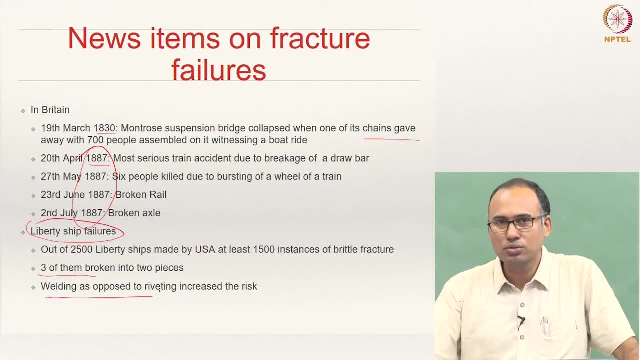 scientific community to pay more attention to the behavior of mechanical behavior, of the structures which have cracks in them And, if at all, there is a crack. now you are required to find out: is this crack okay to live with or not? And that is how the birth 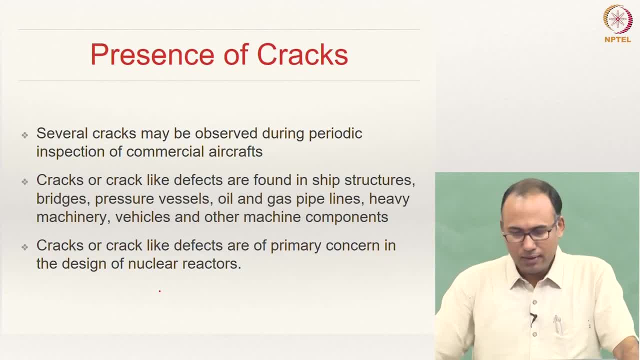 of fracture mechanics took place. So you have presence of cracks in almost every body. Usually the aircrafts- commercial aircrafts- are inspected periodically for these cracks, And some several times. you may observe several cracks during periodic inspection And you will decide whether you need to fix the crack or not. So if I tell you that there is a 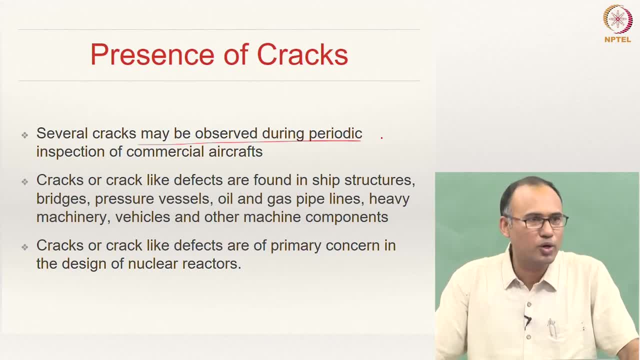 crack in on the aircraft that you are about to board. but it is okay, you can board. What will you do? You better cancel your trip, right? But the beauty of this field of fracture mechanics is that it can actually predict. I have a crack and I know what is the load. 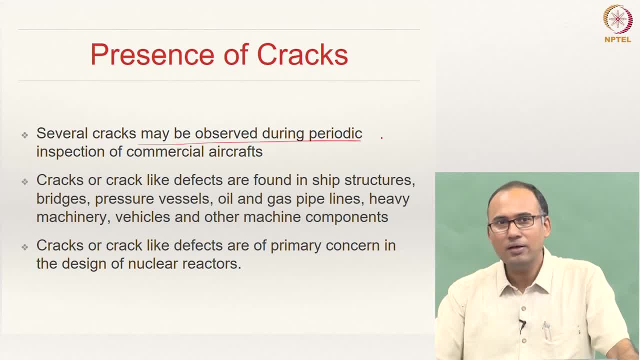 this guy is going to be subjected to, Then one can actually predict whether the crack that is there is going to be a dangerous crack or not, or that is going to be active, or is it going to grow or not. So if you are able to predict that, then you can say that okay. 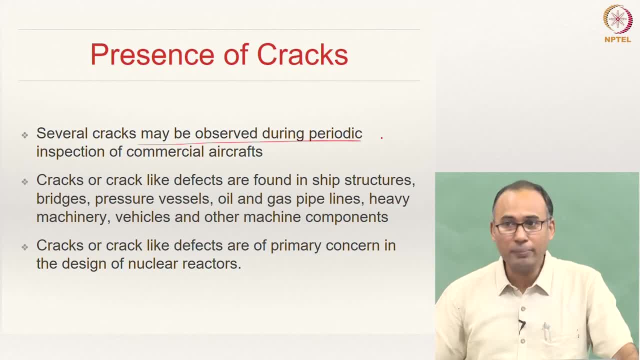 I can have a little bit more life to this component before I can actually fix it. So these periodic inspections are extremely critical. So for components of this kind, so aircraft structures, so they observe using some sort of non-destructive testing right? So ultrasonic waves, guided waves people send to the structure. 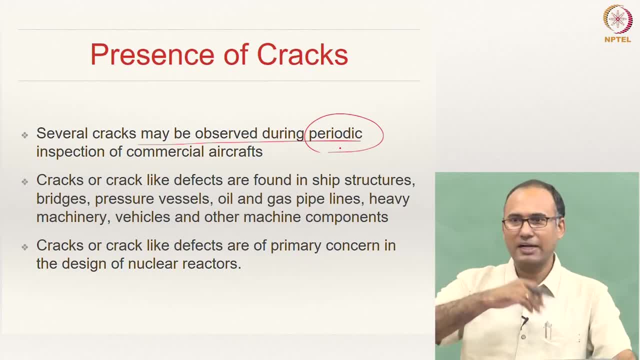 and then see if there is a crack, then the ultrasonic guided wave reflects and depending upon the speed, you know the speed of sound in the material right, And then you can see what is the size and position of the crack and then you can sort of figure out whether 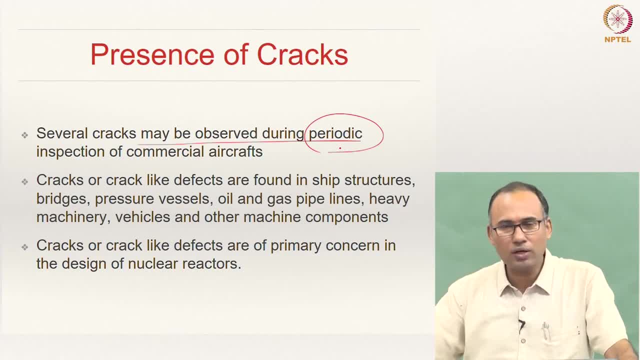 that is a critical crack, or not, right? That is something that one. there are several startups at IIT Madras which uses this technology to study, for instance, pipelines- very important problem, right? You probably heard of detect technologies and so on, right, All these are startups from your seniors, right? So we? 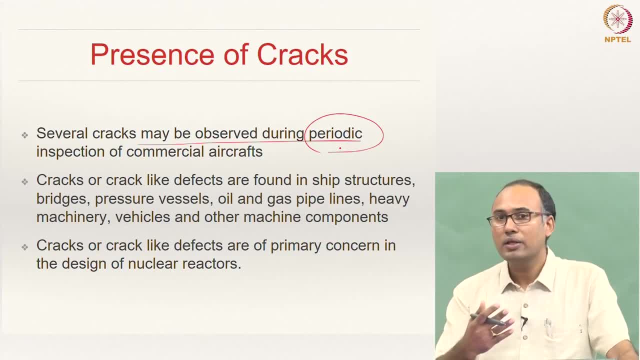 have. so you have. these are the kind of technologies that one can use. So these are called non-destructive testings, because you do not have to spoil your specimen, which you are testing, right, And you also have these cracks, or crack like defects. When we say crack, not all of them. 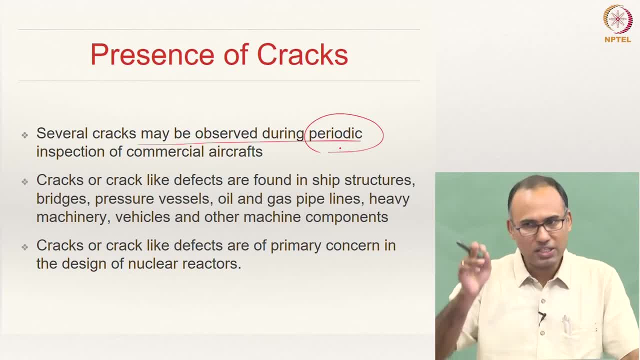 are cracks. some of them are crack like defects, like notches or these things may eventually become cracks, okay, or holes and so on. They are usually found in structures like ship structures, bridges, pressure vessels, oil and gas pipelines, heavy machinery vehicles. 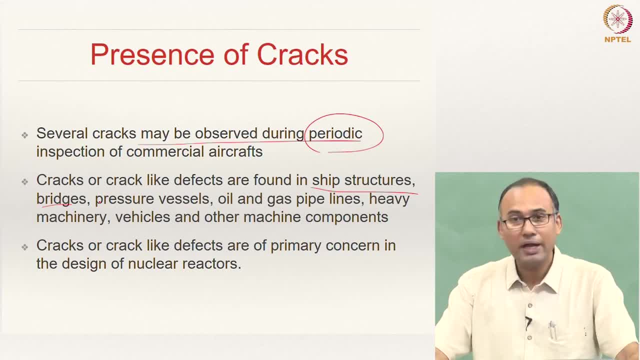 automobiles, any grounded vehicle, ground vehicles and several other machine components, And no matter what, you will always have these defects, As we have been discussing. defects of all kinds at all scales are basic part of every structure. You cannot say that I. 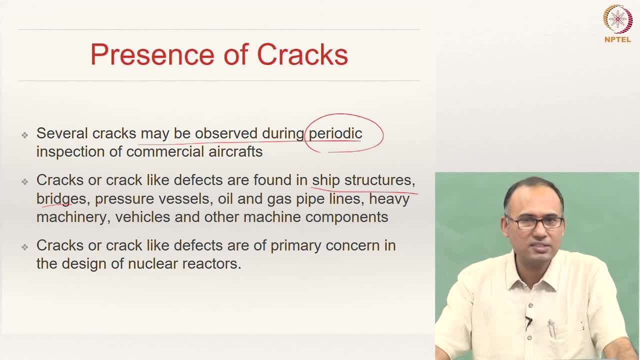 will not use a structure which has a small crack. It is probably okay to use it, provided you know that the crack is not a not going to grow. And one of the major concerns, or primary concerns in the design of nuclear reactors is also this crack, or crack like defect, because this is this- can actually be very catastrophic. 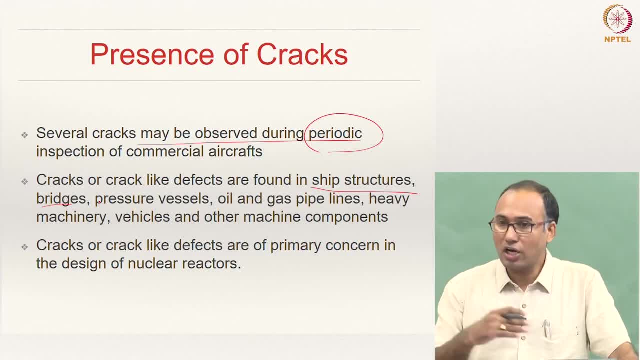 right, If there is a crack in a nuclear reactor, it is not only the fracture of the reactor or breakage of the reactor, but what happens afterwards, right? the radiation effects and so on. So the fracture mechanics principles are extremely important. They are the ones that 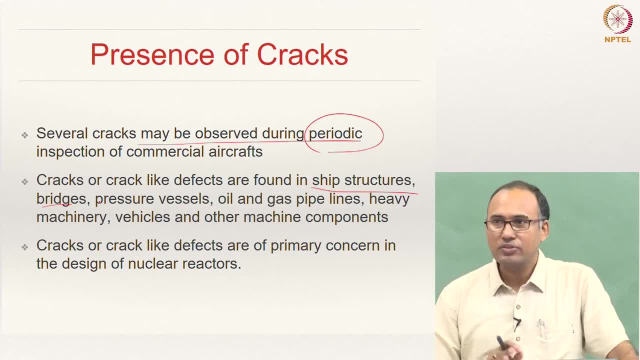 are most important, right. So we take one of these and the other one is the fraction of the reactor. So this is one of the major concerns, or primary concerns in the design for designing these kind of critical structures, whether it is an aircraft or a nuclear reactor. 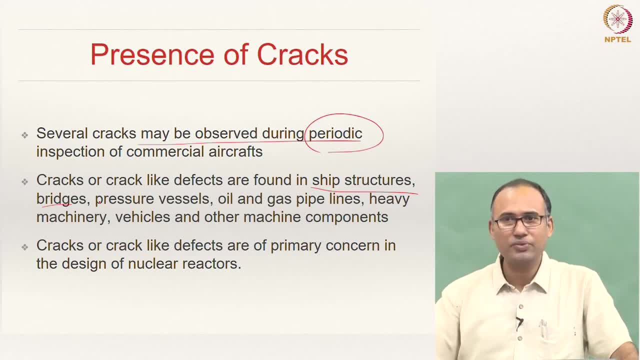 or an automobile. In some places they are. it is extremely important that you should design the structures for fracture Before- excuse me, before the evolution of fracture mechanics or before the introduction of fracture mechanics, people were only designing structures based on strength and deformation. 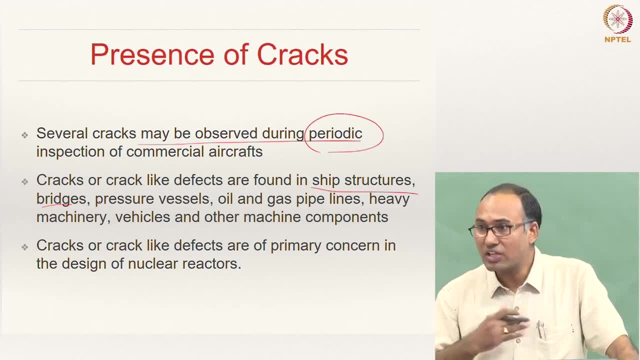 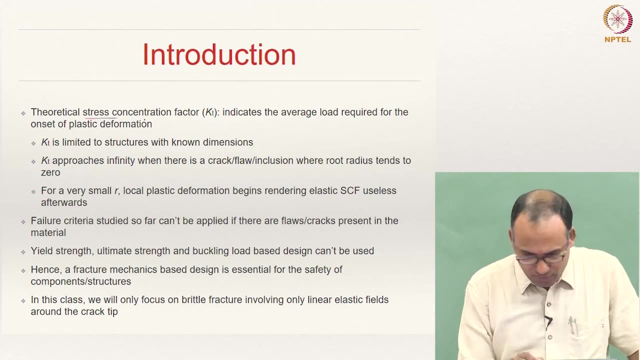 what we have done until last class. Only after the evolution of fracture mechanics it was possible for us to design structures for fracture, And in the last class we have actually talked about something called stress concentration factor. Why So, when you have a crack? 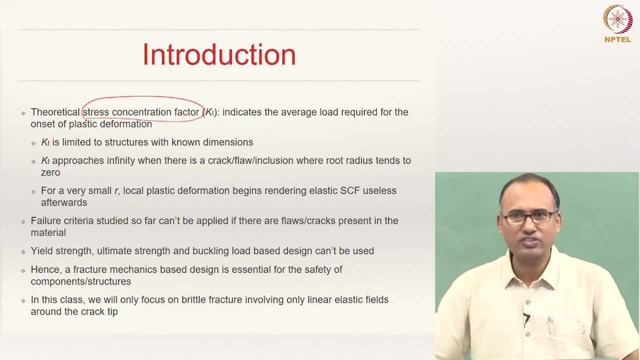 When you have a crack, like defect, a hole, an elliptic hole in the. we have seen the example of an elliptic hole. We have also seen the example of a notched bar and so on. there we have defined something called stress concentration factor. 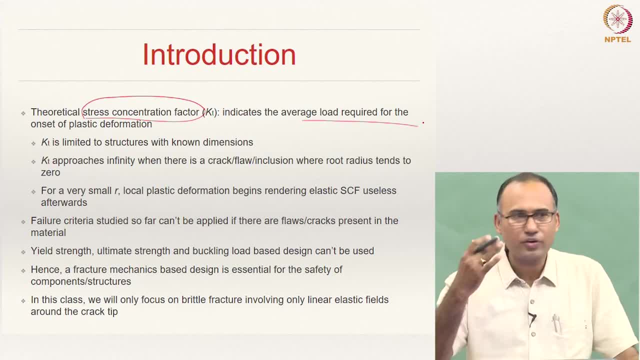 This basically indicates the average load required for the onset of plastic deformation, right? Because we have used it for ductile failure. So when we are comparing in the design process, we are comparing our stress induced is equal to stress concentration, Right. 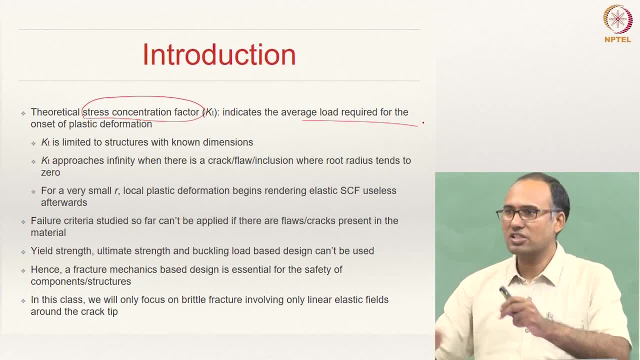 Stress concentration factor times the nominal stress that the far field stress that you have applied, Okay, And hence Kt is limited to structures with known dimensions, because you should know the dimension of the. so you probably have, you probably remember our charts for Kt, where 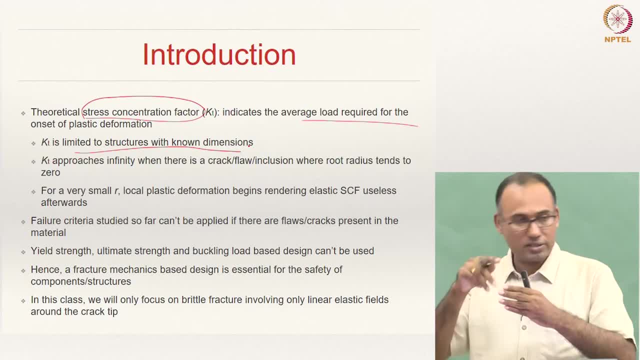 you have capital D by small d ratio and small d by small r by small d ratio. Depending upon these values, you will have different Kt values. Right, And as we have seen, Kt approaches infinity when, the when. so we have seen that in the case of an elliptic. 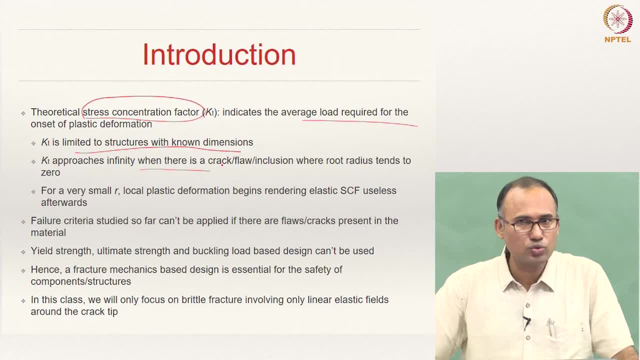 crack. So we have seen the stress concentration factor is 1 plus 2 times C by B or C by A, whatever. But if you can, you can also write that in terms of the curvature, Right, When you do that, the curvature, if the curvature goes there, you, the curvature goes into denominator. 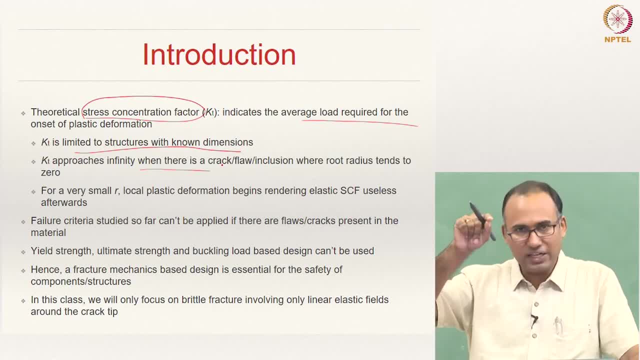 And when the sorry The radius of curvature goes into denominator, When the radius of that guy becomes 0, then you have a sharp crack, Then your stress stress will be. stress at the tip of the notch will be infinite, as opposed to when we have seen a elliptic crack. we have seen that it is the stress concentration. 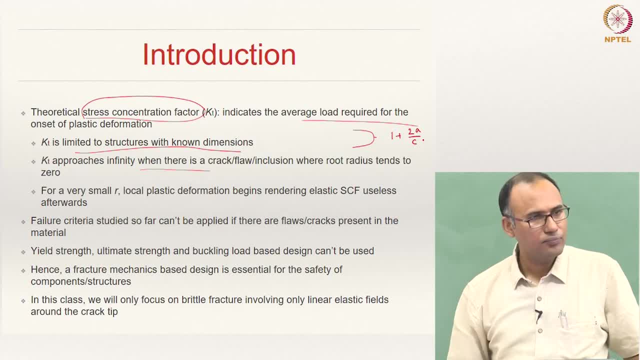 factor is 1 plus 2, A by C, Right? Well, if this happens to be a sharp crack, then this becomes infinity, Because you can actually write this in terms of a square by r, and r is the radius of the crack. 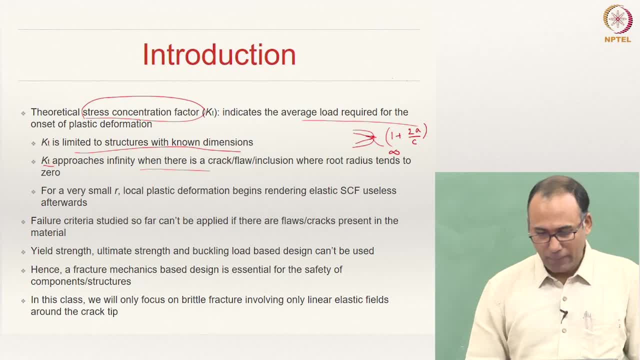 So Kt, the stress concentration factor, approaches infinity when there is a crack, slash, flaw or inclusion where root radius tends to 0. So our stress concentration factor is predicting infinite stress. but real materials will not have infinite stress because there are some limitations. we will see what are there. 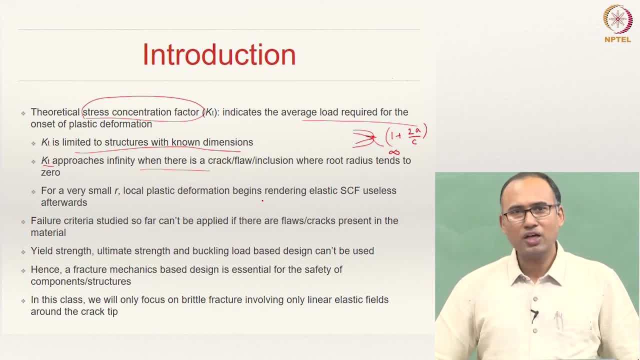 The reason why real materials will not have infinite stress is that because you cannot have exactly infinitely sharp crack. Because if you zoom in locally, first of all, if you have a really a sharp crack, even we see the slightest of the externally applied load, you will impart plashy deformation here. 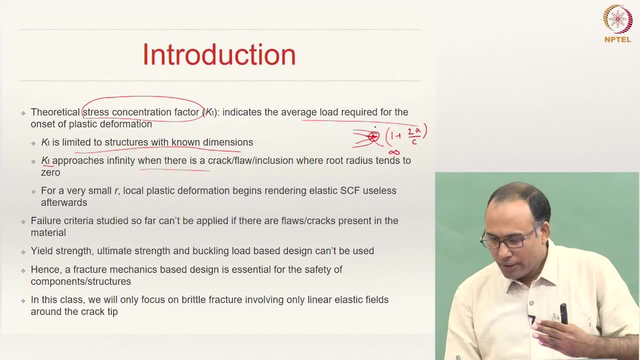 The moment you have plashy deformation, the stress state around the crack tip will make the crack blunt. The moment you have a small force, it will already get into plashy deformation and, as a result, your crack becomes blunt and, as a result, you cannot have infinite stress. 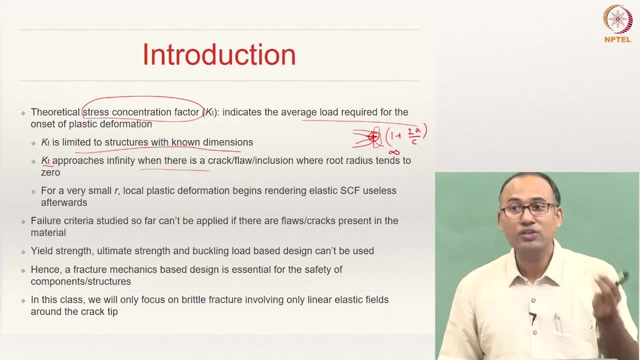 That is one thing. And the second thing is you cannot have 0. 0. Radius, because at the atomic scale your radius cannot be smaller than the atom radius. so, no matter what, you do not have atoms of 0 size. So, no matter what, you cannot have a atomically sharp. 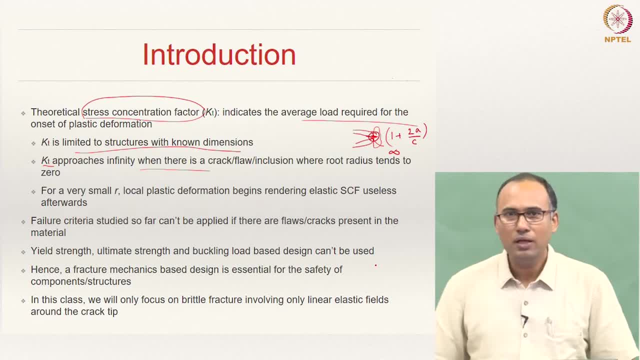 So you will always have some radius that you need to work with and hence real materials will not have. mathematically it is possible, but reality is far from what we describe mathematically. Okay, So what we have- failure criteria studied so far- can be applied if there are cracks. 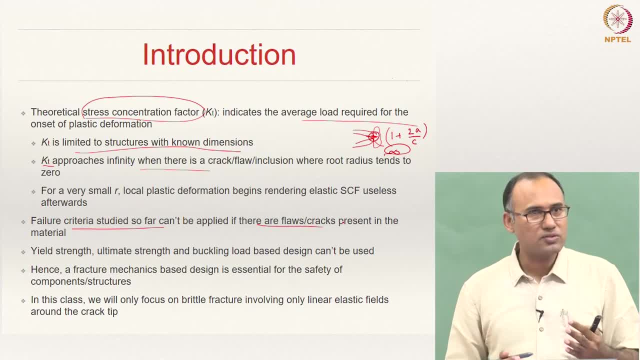 or flaws. as we have already discussed, the one of the important assumptions when we are writing static failure theories was that there is no, there is no crack present in the material And hence you cannot base your design on yield strength or ultimate strength. and there is also another failure mode in materials called buckling failure, which we have not discussed. 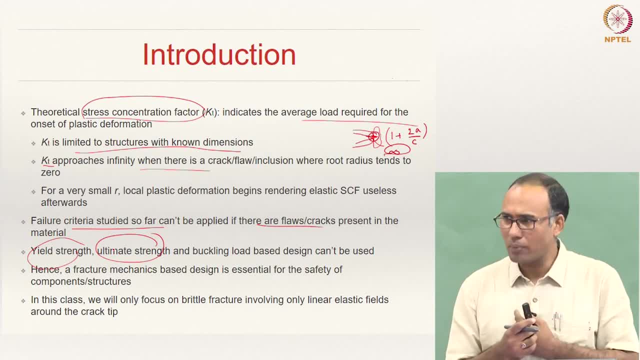 but in your strength of materials class you probably have done column buckling right, Have you done? Some of you have done, some of you have not. So if you have a column like that and if you apply an axial load, then this column- 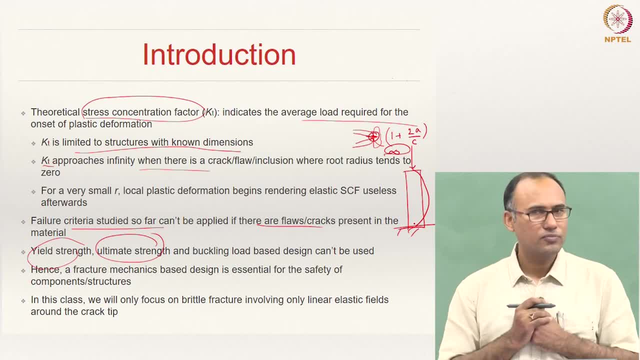 can at some load that column can buckle like that it will. you are applying an axial load and column buckles out of it. the displacement is coming this way. Does that make sense? It makes sense, Isn't it violating Newton's law? 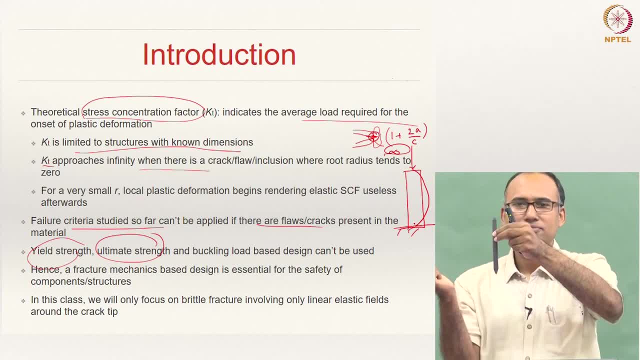 If you are applying a load in one direction, how can you have displacement in the other direction? Is it violating Newton's law or not? Think about it. Okay, So you can have failures like that. that is also not acceptable, because you have designed. 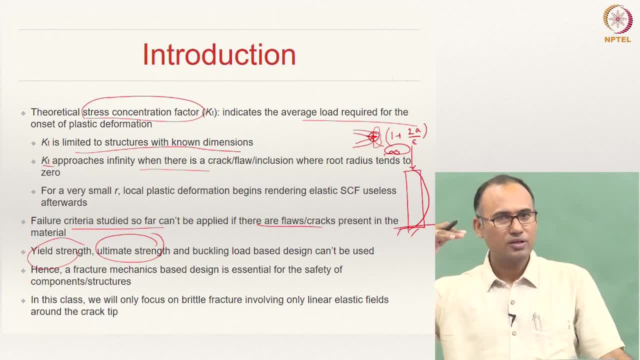 this column to be straight, And if it bends like this, it is not going to serve the function for which it is designed. So you also need to think about when you have compressive loads in the members. you also need to worry about buckling along with other failure modes. 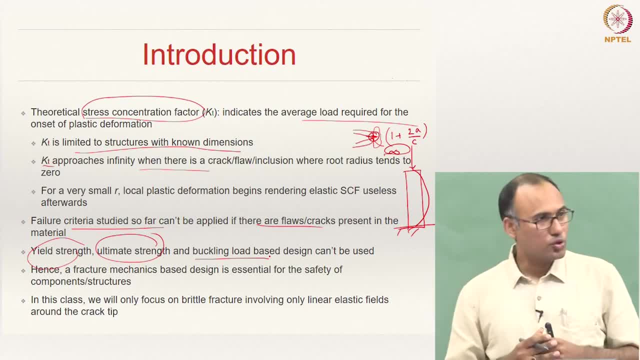 Okay, So now, the moment you have cracks, you cannot base your design just on these things. you should be worried about failure. So hence, a fracture mechanics based design is essential for the safety of any components or structures that we are defining, and in this class, we assume that the stress state 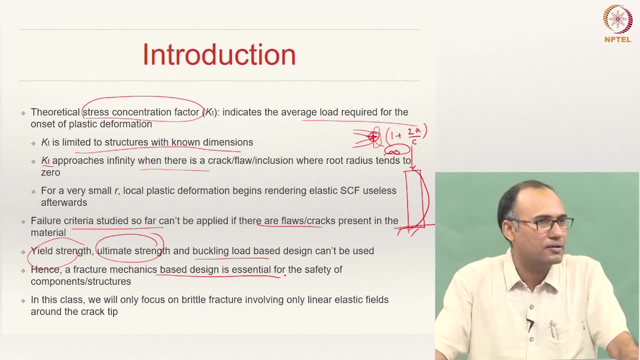 around the crack tip is only purely elastic, linear elastic. We are not going to consider any plasticity whatsoever because that is again that involves other complications. So we are only focusing on stress fields in this class. Okay, So stress fields around having linear elastic fields around the crack tip and such an area. 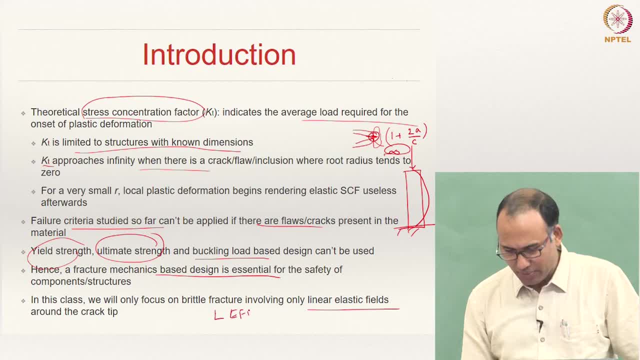 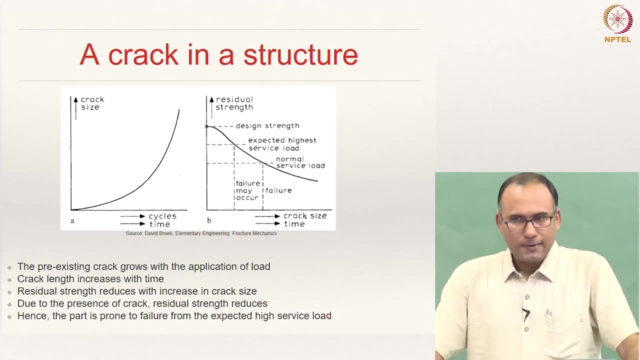 of fracture mechanics is called linear elastic fracture mechanics- LEFM, And if you have plasticity around the crack tip, then it is called EPFM- elastoplastic fracture mechanics. Okay, All right, So when you have a crack, Okay. 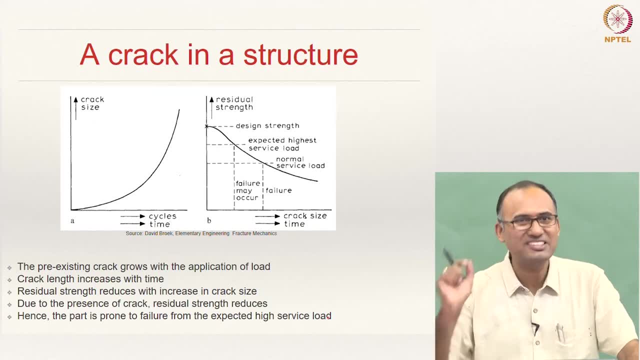 In a material. So you have a pre-existing crack. So the figure on the left hand side is actually showing you: on the y-axis you have crack size. on the x-axis you have time or number of cycles of load. So you are actually applying a cyclic load, time varying load. 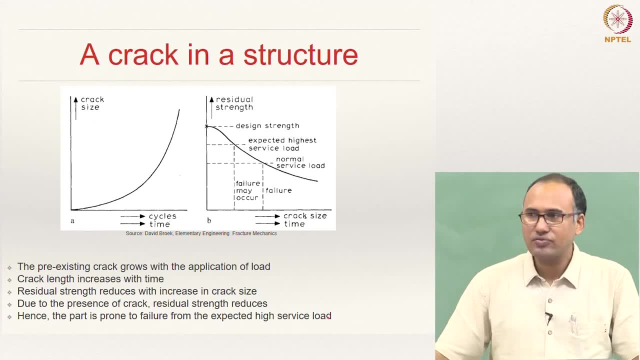 Then the pre-existing crack grows, as with the application of load, as you increase the load that the pre-existing crack can actually grow, or with the time it can grow. So as a result, the crack length increases with time. Initially you may have a small crack, but because of the application of the load, the 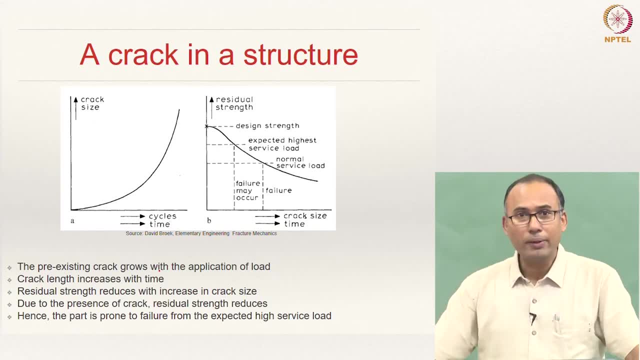 crack length increases with the function of time. The moment you have a structure with some pre-crack, it will have some strength. That means the load carrying capacity. The moment the length of the crack increases, what happens to the strength of the structure? 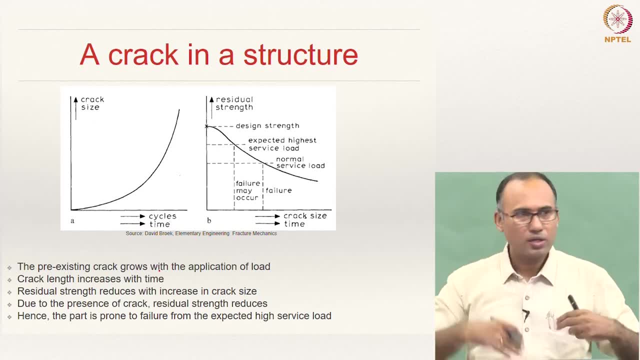 It reduces That, that the residual strength comes down as you crack length, as you crack length, as you crack length. Okay, So the figure on the right-hand side is actually showing you when, my when- there is no crack. 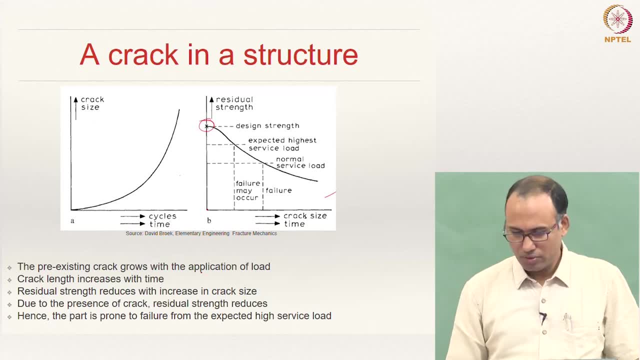 this is my design strength Right. So at 0 time there is no crack, or you may have one crack and then that has some strength. like that: Right As my time is increasing, my crack length is increasing. Right Here: as the crack length is increasing, my residual strength is decreasing. 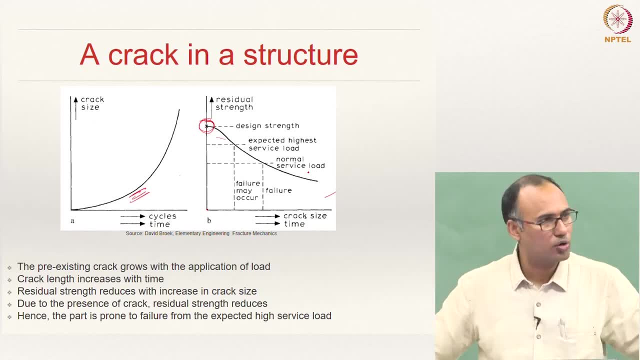 Because the length of the crack is increasing, The amount of available area to resist the load is decreasing, So the part is prone to failure. So this is the design strength of the part, But because of the fact that you are applying the load, the length of the crack is increasing. 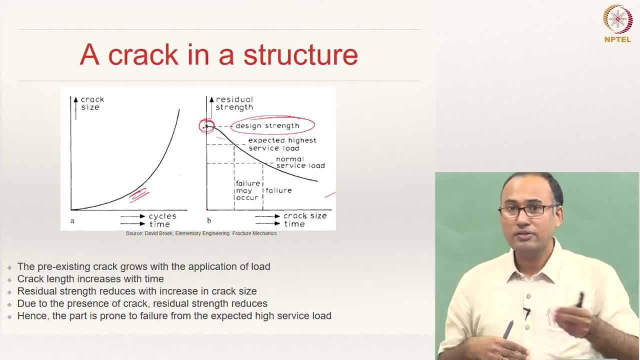 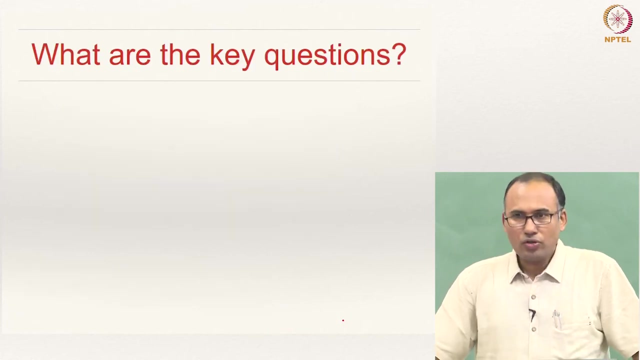 As a result, the residual strength is decreasing and hence the part might actually fail before it reaches the design Right. So there may be a premature failure of the component than the expected high service. Okay, Alright, So what are the key questions to ask? now understood, having understood how a crack 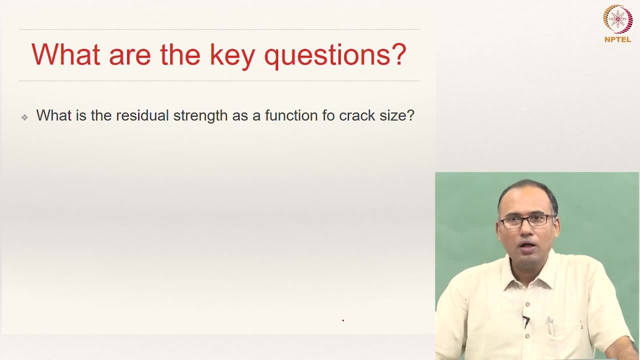 behaves and so on. We said: as you increase the length of the crack, the residual strength reduces of the component. So what is the residual strength as a function of crack size? Can you actually relate these two things? And the second question to ask is what size of a crack can be tolerated at the expected? 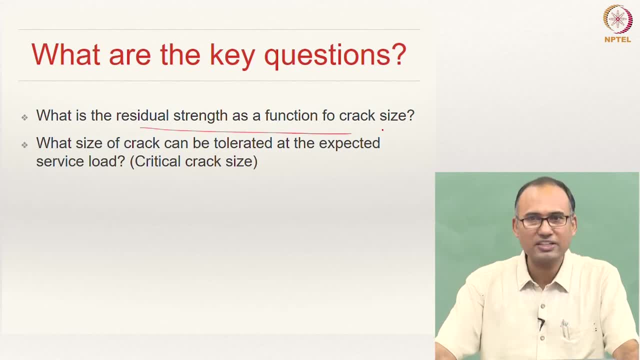 service level. Right, So if I have certain size, you say that if my load applied is such and such, if it is below certain threshold load, then the crack may be okay to use, Right? Yes, It may be okay to have the crack there, because the crack is not going to grow. 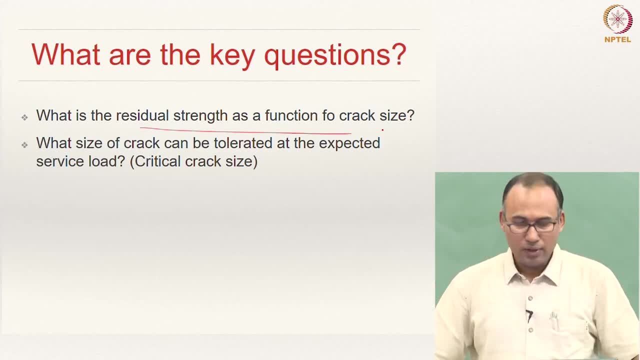 The material is still able to withstand the load that you are applying. So the question to ask is: what should be the size of the crack? So what is the critical size of the crack that can be tolerated at the expected service level? 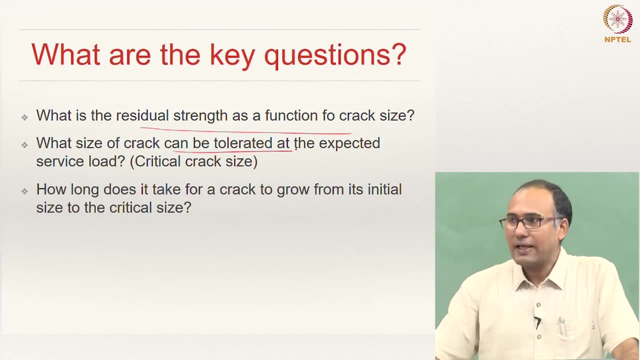 And then, as we have discussed with, as a function of time, your crack grows. So the question to ask is: how long does it take for a crack to grow From its initial size to the critical size? So you know, you have a component, and let us say I have a crack here and I am applying. 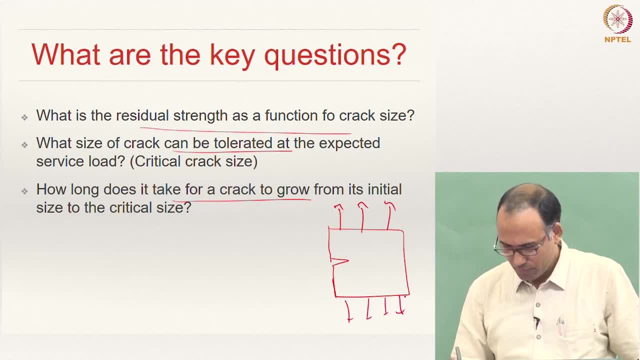 or let me say I have a crack here. I am applying a load for filled load. This crack length is, let us say, 2a. Now the question is: when applying for filled load, How long does it take, Because this is a time varying load. f sigma is a function of t. 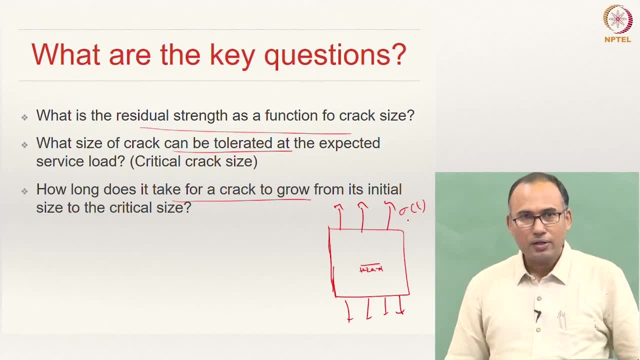 So how much time do I need to wait so that the length of the crack increases to a critical size? What do we mean by critical size? Once you reach the critical size, the crack zips through. Crack suddenly zips through the entire structure. 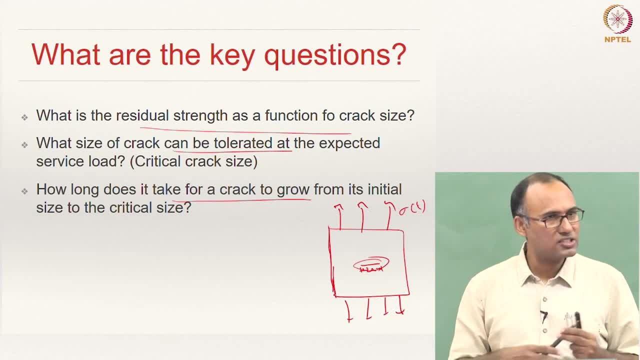 That means you do not have any time. The moment it reaches critical size, it will grow. Okay, It will break in a brittle manner. Until then you do not have a problem. So what is the time? How long does it take for the crack to grow from its initial size to the critical size? 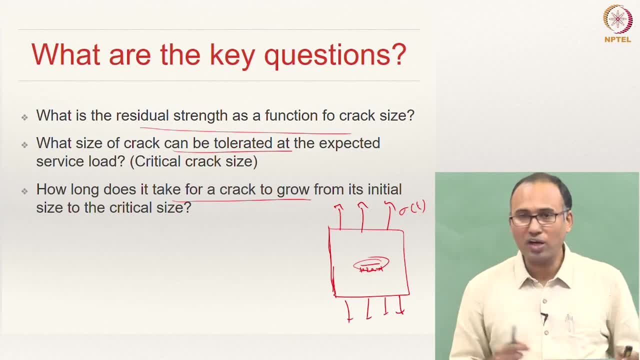 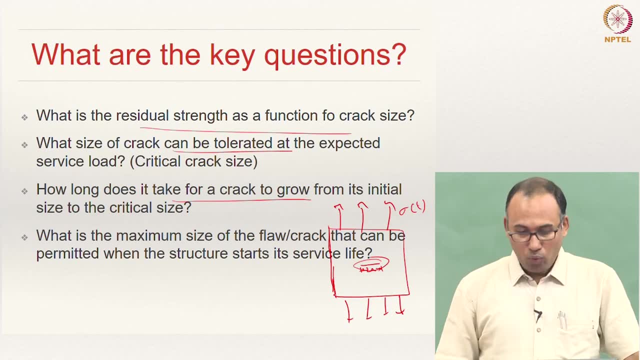 And what…? So, given a structure and given a load, what is the maximum size of the flaw or a crack that can be permitted when the structure starts its service load? It did not…. You have designed the structure, but you found a crack there. 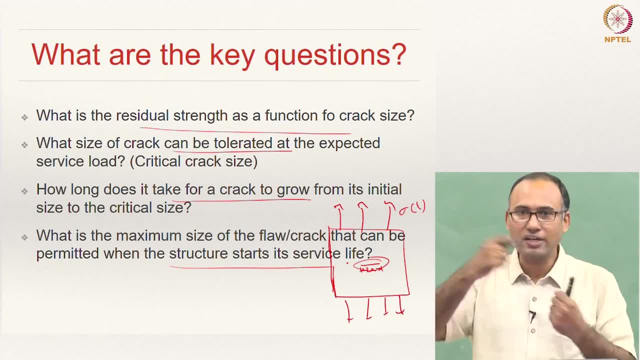 And what is the maximum size of the crack that you can permit when it is starting its service load. That means you know what is the maximum load that this guy is going to be subjected to. If you know the load that is this guy is going to be subjected to, then you can say that. 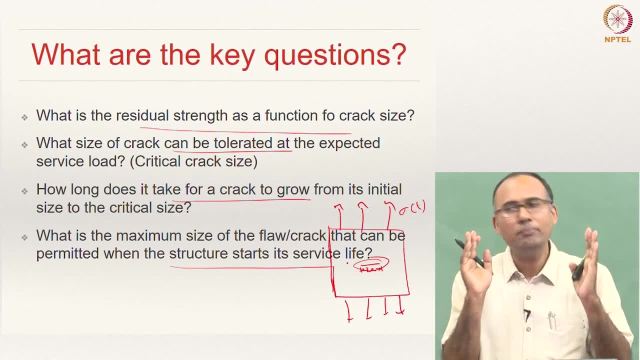 okay, this size of the crack. if it is 1 mm, I am fine. If it is 1.5 mm, also fine. If it is 2 mm, you have to stop Right. So… You have a component. 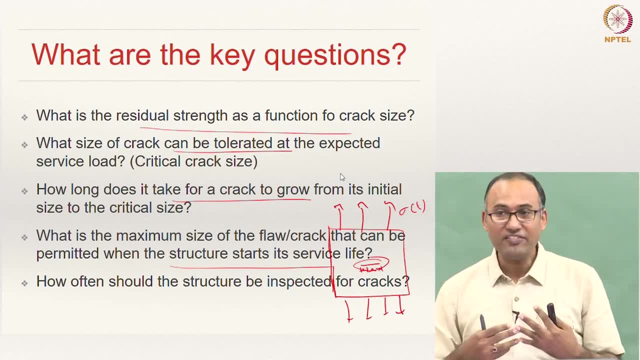 For instance, take the example of an aircraft. You have cracks to begin with And you said that okay, for that service load, the crack is fine, This is not a dangerous crack. But then we know that as time progresses, as aircraft makes several trips, your crack. 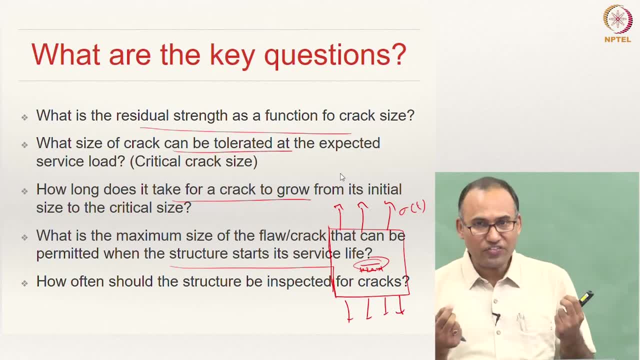 is going to go grow in size. So then you need to verify whether… Okay, Your aircraft has cracks which are critical, But then will you do this check with each and every flight? Then airline companies will be making lot of negative profit. 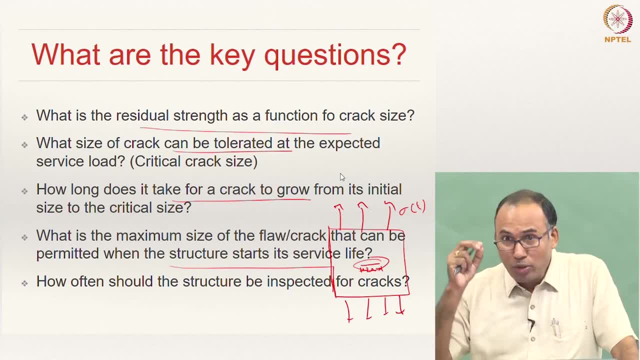 Right, So you should be able to prescribe how long should I wait from one check to another check. What is the time period? Okay, What is the time period from one check to another check, Or how often should I inspect the structure? 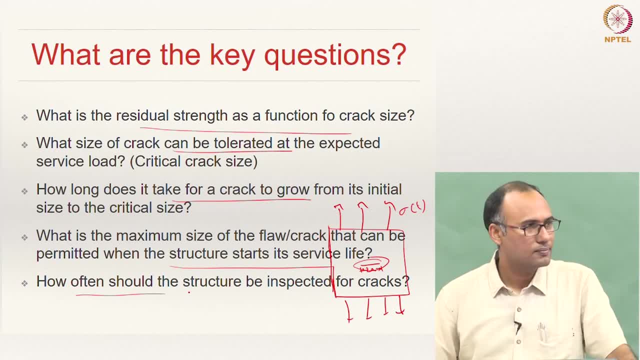 Because you know, by knowing the… See, when the aircraft is flying, you know the load history. It is not going to be constant load, Is not it? When the aircraft is subjected… When it is flying, suppose if it encounter… If it is a smooth flight, no turbulence whatsoever, then we know what is the load history from. 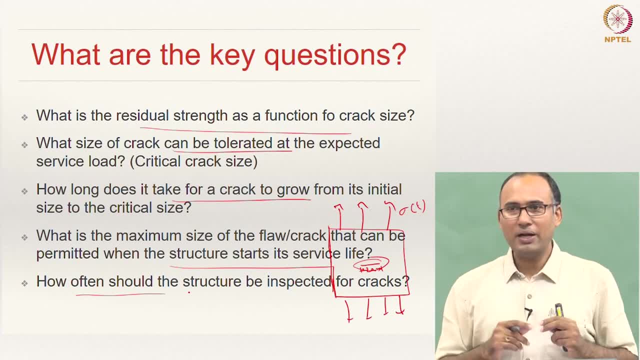 the time of takeoff to landing. Okay, That is the study, But let us say you have a…. The aircraft encountered some severe turbulence, So this is not your service. load Right: You have some load which is beyond what you expect. 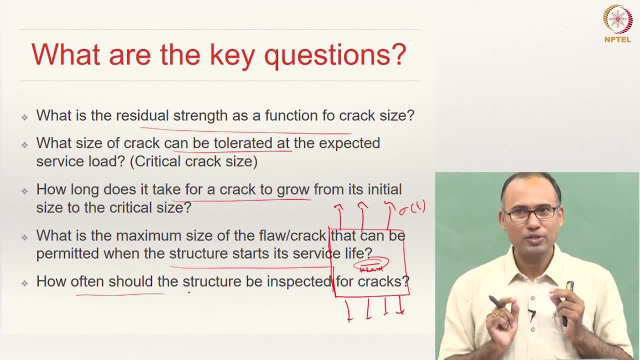 And then you need to take that into account. if that there is serious turbulence, or okay, with acceptable turbulence, Then based on that you prescribe how many times in a month or two months you need to send the aircraft. Okay, How many times you need to send the aircraft for evaluation? 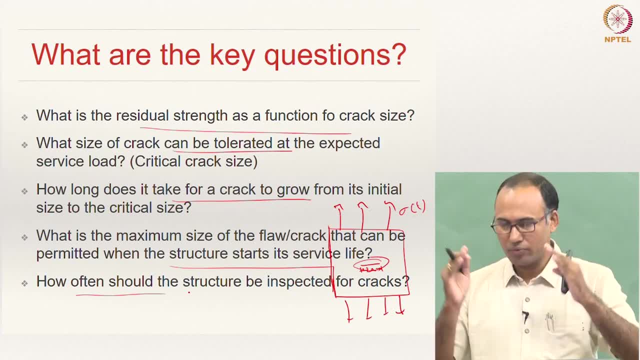 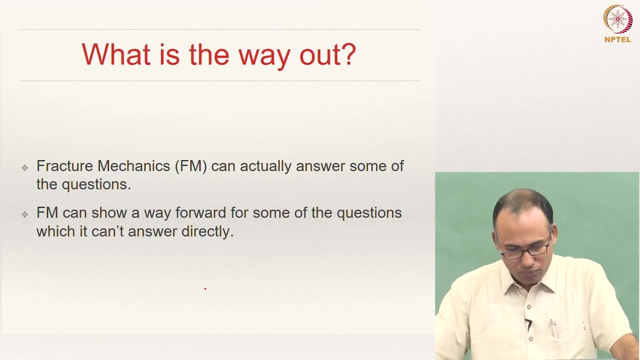 Whether the crack sizes are well within the limit or not. So the time also should be prescribed. These are the questions that one need to answer when we are designing something for failure or fracture. So the questions that we have asked so far did not even arise when we are doing the design. 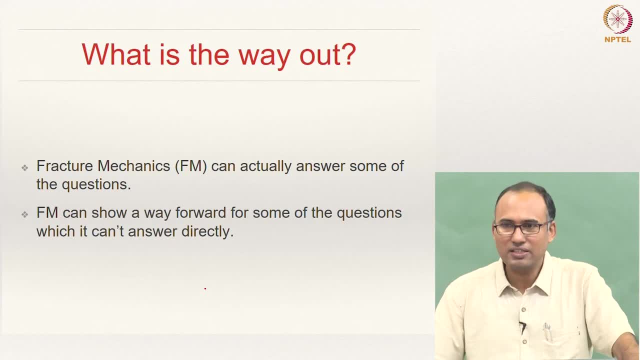 based on static failure phase, Is not it? Because there was no crack to begin with, But then, in order to answer the questions that we have just now posed, fracture mechanics will help us. You can actually answer some of the questions, not all of them. 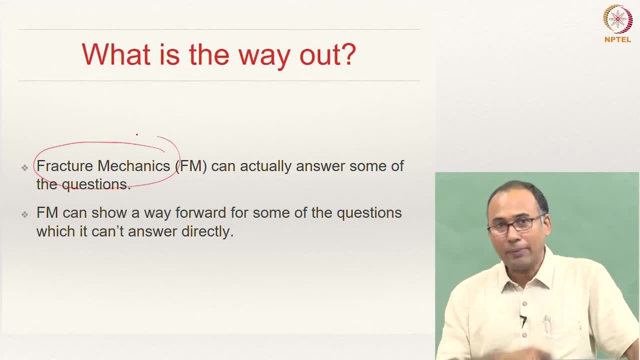 And for some other questions for which it cannot give you direct answers, but it can show you a way to find the answers Right. For some of them it can answer And some of the questions you probably will get a direction on how to find the answer. 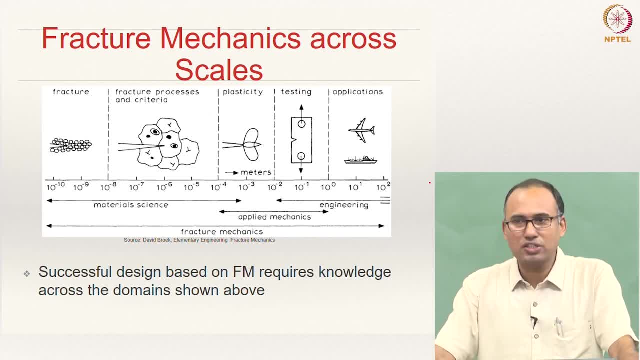 Alright, So you can study fracture behavior at different scales And many times, as engineers, we are interested in designing structures at this scale for safety against fracture failure, Right, But the microscopic mechanism for fracture starts at this scale, But you do not necessarily study how a crack is propagating by looking at an FCC crystal. 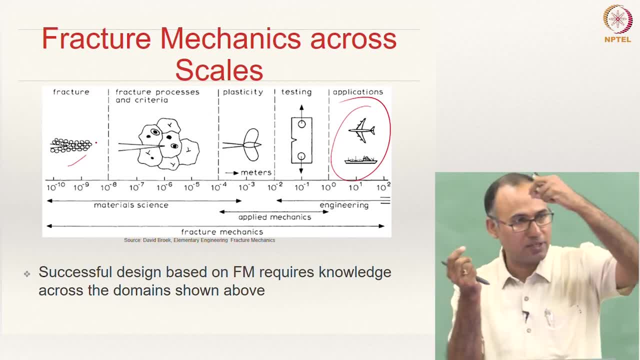 structure and each and every item and how the crack is propagating. That is the job of somebody else. If you are designing structures, components, at that small length scales, then you need to worry about those mechanisms, Right, So you, most of the times, we develop theories which would homogenize the information that 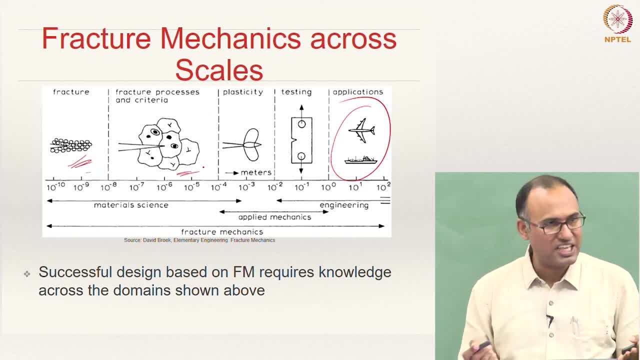 is observed, or the mechanisms that are observed at these scales to a reasonable length scale at the laboratory testing scale, And then based on this information these guys will be designed. But the information that we are prescribing here will actually come from the microscopic mechanisms happening at these lengths. 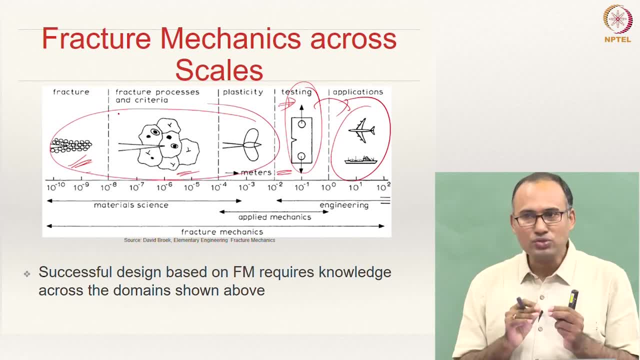 But we will not use those phenomena directly, but indirectly through some parameters. Alright, Alright, But however, you need to know what is happening at the microscopic scale, How So basically, fracture means what Breakage of bonds between atoms, Right? 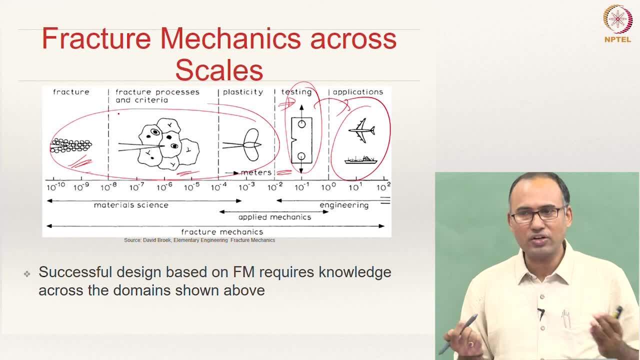 So you are creating two new surfaces. Until then there was no new surface and then the moment the crack gets open, crack propagates. there was no new surface. There was no new surface. now you have created a new surface. That means you have broken the bonds. 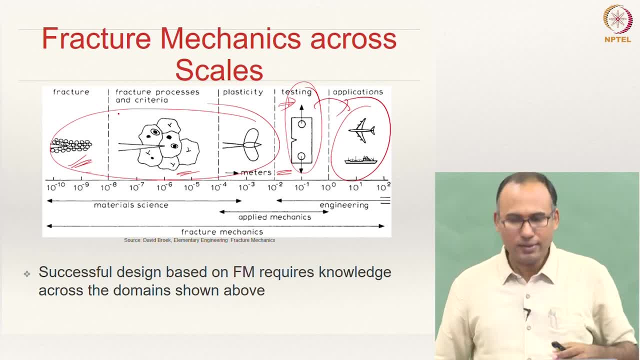 Right. So that is the fundamental mechanism, But what is responsible for that is something that will become clear, depending upon the kind of the material that you are using, depending on the kind of the microstructure that you have for that particular material, and so on. 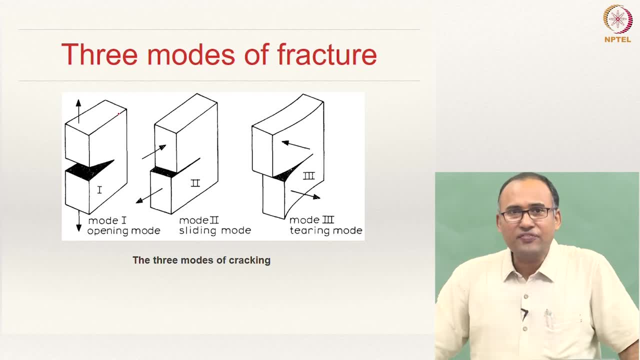 Okay, Alright. So when we are studying fracture, you have three modes of fracture: Mode 1, mode 2, mode 3.. So mode 1 is also called opening mode. So you have a component, and then this is: let us say, this is your crack face and the 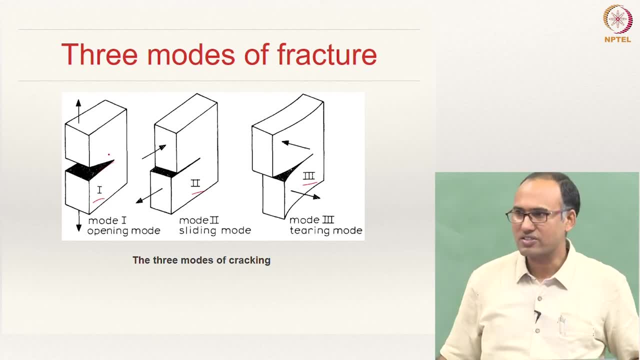 load is applied perpendicular to the crack face, Okay, And then, because it tends to open the crack surfaces, it is called opening mode, And mode 2 is called opening mode, Okay, And mode 3 is called shearing mode or sliding mode. 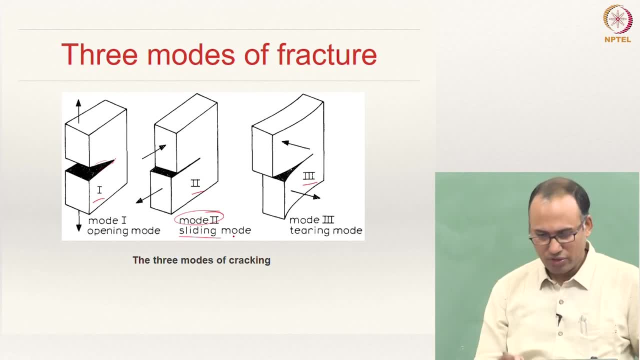 Right, The load is parallel to the surface. you can see, But in the plane. Okay, And now the third one is like tearing mode, mode 3.. In this class we will mainly focus only on mode 1, but if you have a fracture, which is 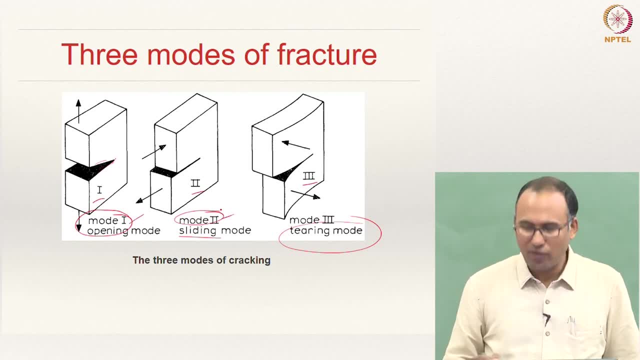 having mode 1, mode 2.. In general you have a fracture. Okay, In general you can have all three modes present. If a crack is expanding or propagating, it is possible that all the three modes of mechanisms are present and such a fracture is called mixed mode fracture. 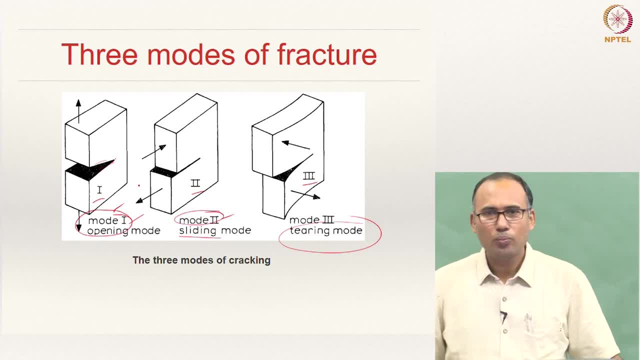 But here we are only going to focus on mode 1 fracture. But if you take a complete fracture mechanics course- several of them are available on this campus- Then you will actually study what is the effect of having a fracture, What is the effect of having mode 2 and mode 3 also alongside mode 1 fracture. 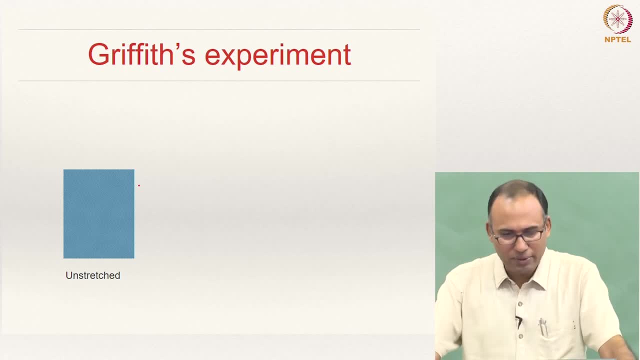 Okay, All right, So this is an interesting experiment. This is what is called Griffith's experiment, So he is the father of fracture mechanics for us. Okay, So he did this very interesting experiment. So you have a sheet of paper, for instance. you can actually do this experiment yourselves. 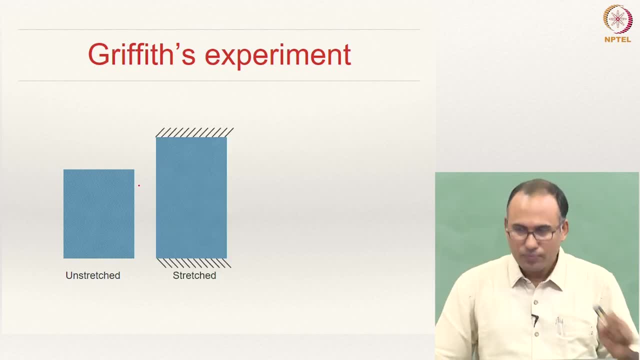 and is unstretched, And then you stretch, you apply certain force and then fix it. That means hold the grips there. Can you do this thought experiment All of you are doing? You can actually do this. I am thinking about only brittle fracture, but nevertheless you can do this using your 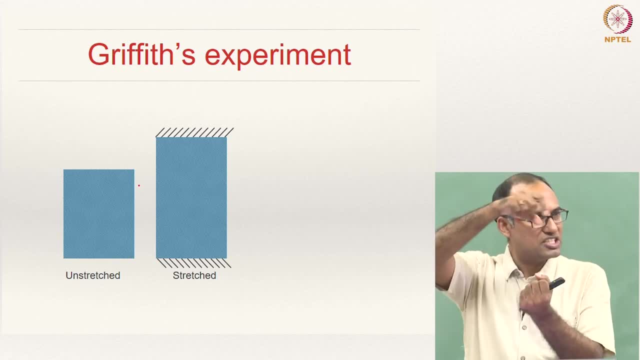 paper or using a polymer sheet. That is much easier to observe. And now what you do is So: you have stretched it And then are holding the grips. That means displacement control. That means you are not allowing any further displacement. Is that clear? 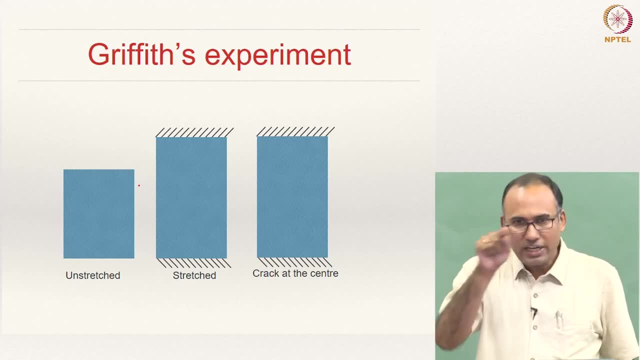 Now use a scissors or a knife and make a small slit in the center somewhere here, So you can do that probably with a paper also. Apply load, Make sure that it is not breaking and hold it. Ask your friend to hold it, as it is very difficult to control the displacement. 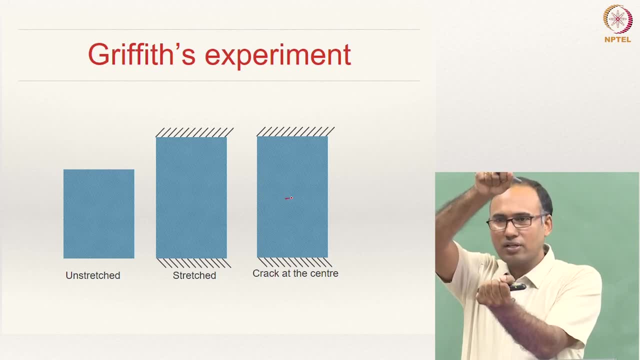 But let us say that your friend is having a feedback loop allowing him or her to actually control that And then make a small slit, maybe using a knife. You can use a knife and small slit. Then what happens is the system will not break. 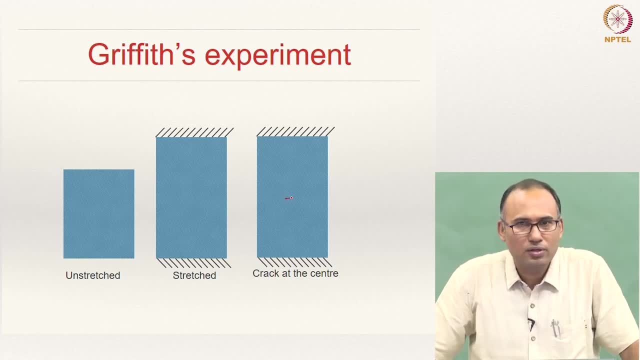 You probably have done this with polythene sheets, and you are a kid. If you have not done that, do it today. And then you ask your friend to continue to hold this and then increase the length of the slit And at some point the length of this crack becomes sufficiently large, after which it 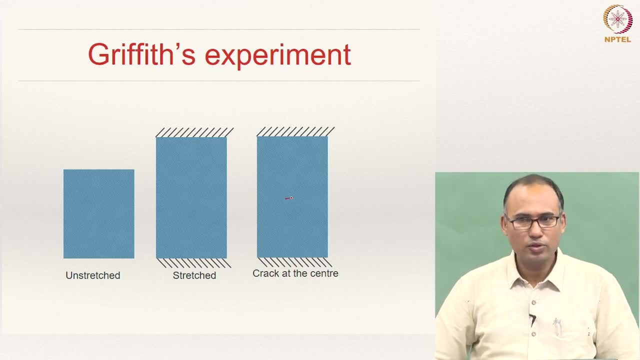 suddenly breaks. You can feel that when you are doing this thought experiment. So let us say that is your crack, And then you calculate: So this is your. let us say the crack length is 2a, And now I am creating what is happening now. 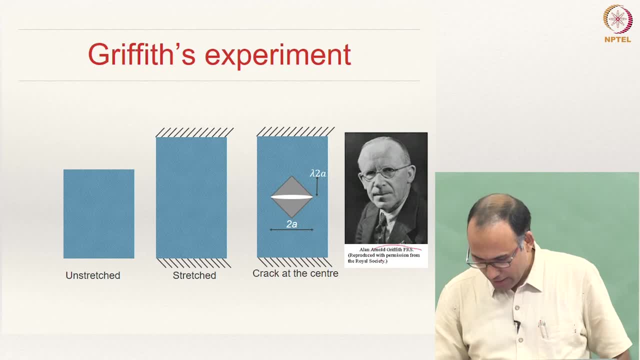 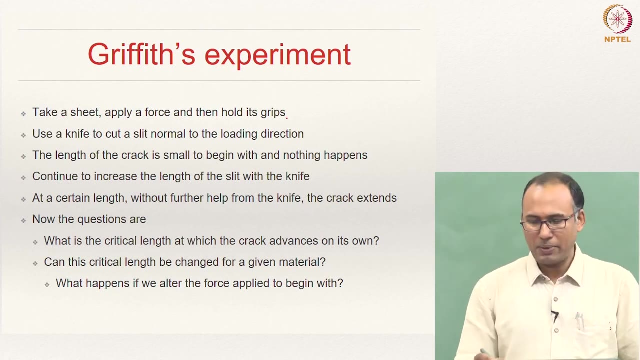 So he is Griffith. He is the one responsible for us to understand design of materials based on fracture. So this is the experiment that we have done: We have taken a sheet, apply a force at the hole and then hold its grips and use a knife. 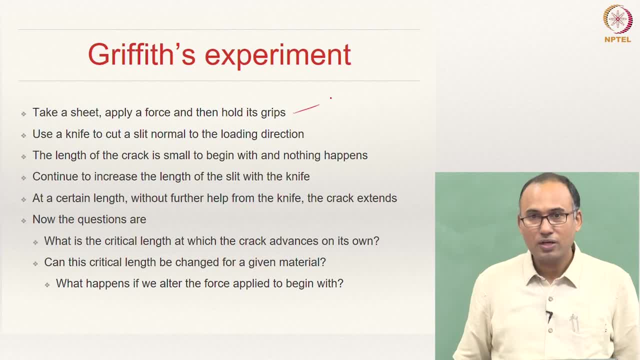 to cut a slit normal to the loading direction, not like this, like that. Do not cut the slit like that, like this. You should cut like this. Only then it is mode 1. Otherwise it is little bit more tricky. 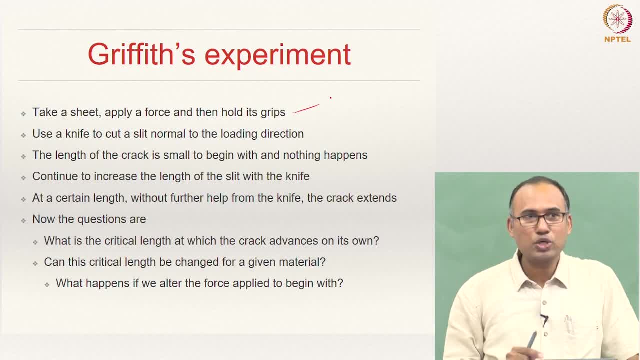 And the length of the crack is in the beginning. Make sure that you do not cut a long slit. Cut a small slit to begin with, So the length of the crack is small to begin with and nothing happens. And continue to increase the length of the slit with the knife. 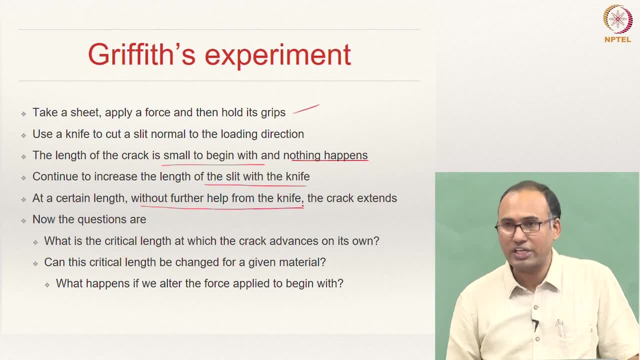 At certain length, as we have discussed, without any further help from knife, the crack extends. Now the questions are: what is the critical length? What is the critical length at which the crack advances on its own? Does this critical length change from material to material? 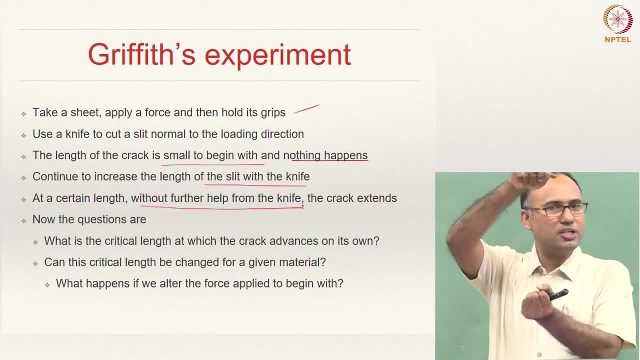 Does it depend on the material? If you take a polythene sheet, polymer sheet, a paper or a metal sheet, does this critical length change? All of them are applied with the same force And if you take a material, does this critical length change as a function of the applied? 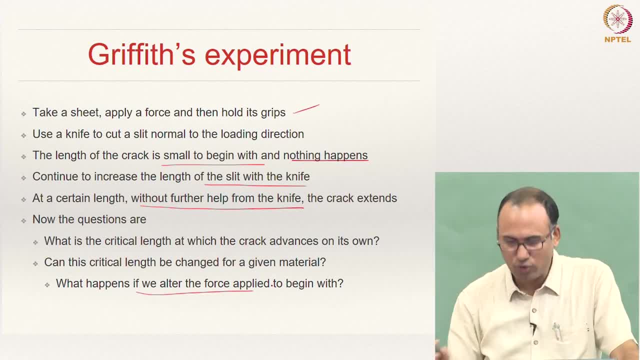 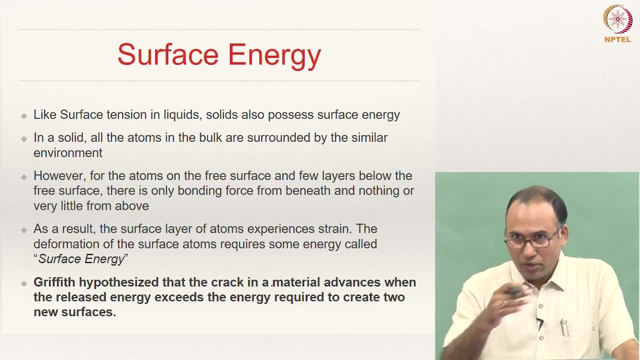 material? What happens if we alter the force applied to begin with? These are the questions that we need to ask, So, in order to understand what is happening when you are cutting a slit to the system. you probably heard of surface energy, like surface tension for liquids. 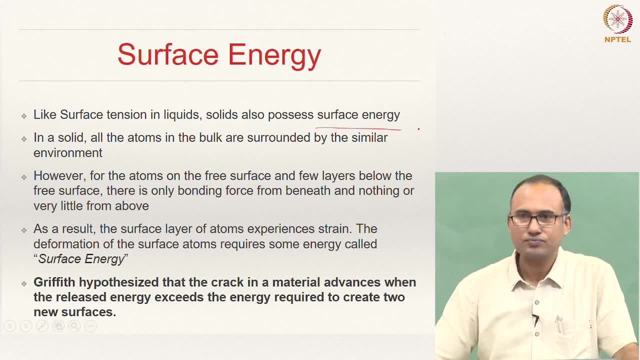 For solids we have something called surface energy. It is very reasonably easy to understand. Suppose, if you take a metal sheet. Suppose if you take a material and look at the bulk, At the bulk take an atom. So if I take this mobile phone and if I consider an atom at the center, not on the surface, 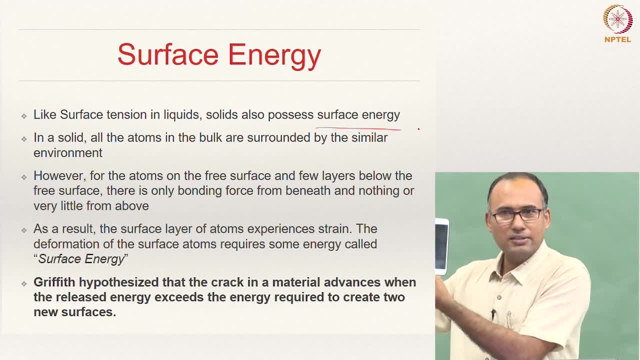 but somewhere in the middle through the thickness, then that atom is surrounded by several atoms. That means it is the bond strength, the bond resistance offered by other atoms is sort of something. But if you go from bulk to the surface, the surface atoms are primarily subjected to the 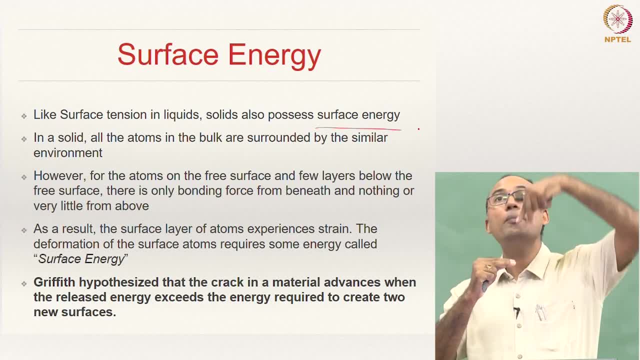 bond forces atoms below them and above them. there is nothing As a result. there will be some strain. They can accommodate some strain because there is no bond above them and the energy associated with that strain is what is called surface energy. So the atoms on the free surface and few layers below the free surface. there is only 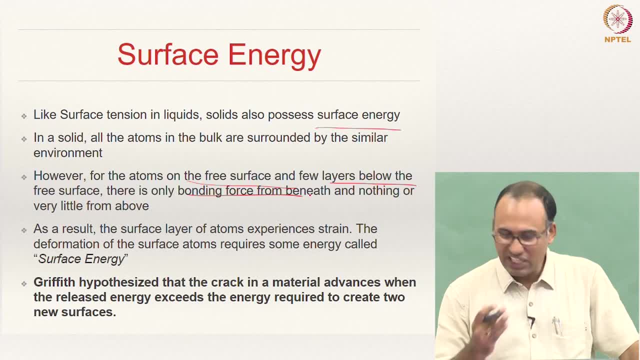 bonding force from beneath and nothing above it. If it is a surface layer, there is nothing above, but one layer below the surface there is a little bit, and so on. As a result, the surface layer of atoms experiences a strain and the deformation of the surface. 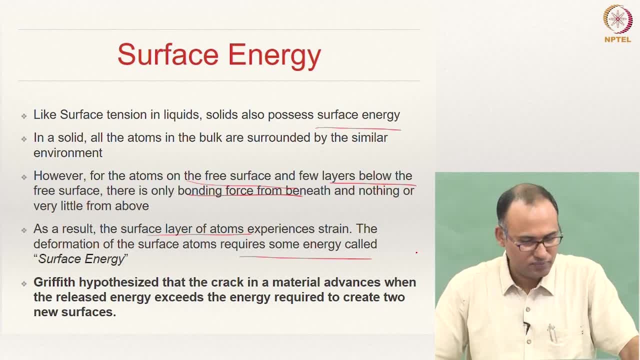 atoms requires some energy, and that is called your surface energy. What Griffith hypothesized from the previous experiment is that the crack in a material advances When the released energy exceeds the energy required to create two new surfaces. What do we mean by released energy? 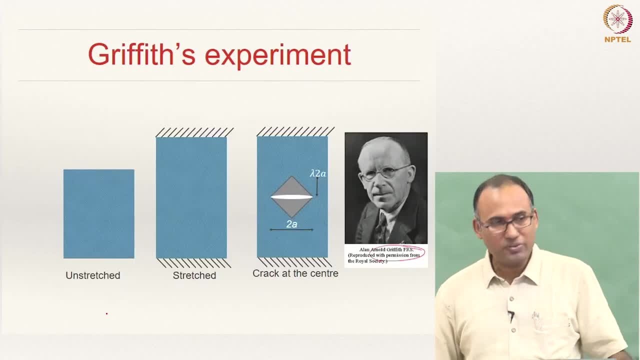 So when? what Griffith hypothesized from this experiment is that when you are creating a slit, you have created new surfaces, right, Where is the? whenever you are creating two new surfaces, you have to provide this additional energy. How did you provide this additional energy? 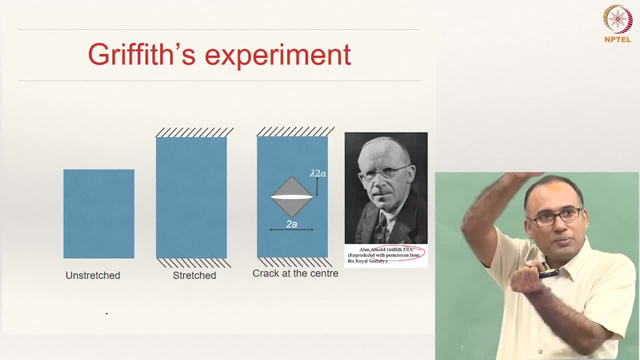 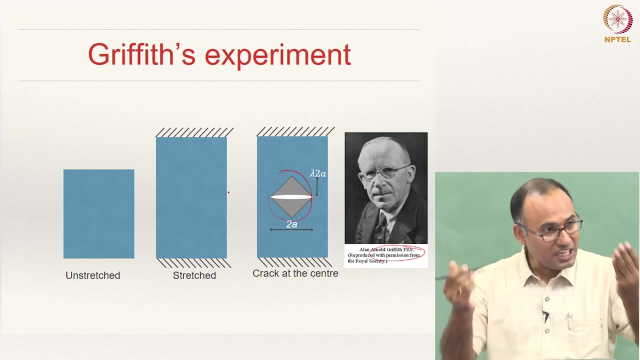 Imagine, when you are applying the load, there is some strain energy stored in the material right Because you have deformed the material. So when you are creating the slit, the material around the slit will release some strain energy and that strain energy will be used for creation of these two new surfaces. 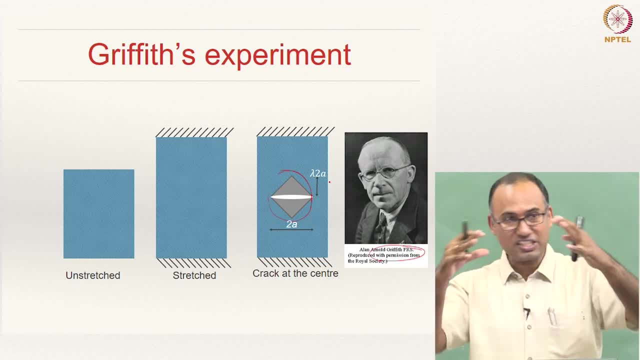 And how much material will? what is the extent of the material that I need to consider? He hypothesized that take two triangles, one triangle above, one triangle below, And where this length is 2a, and he says that this will be lambda times 2a. 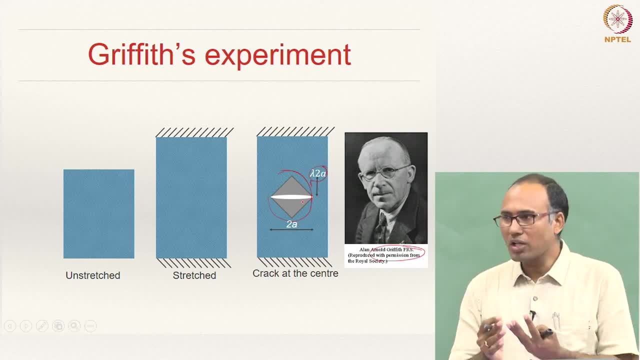 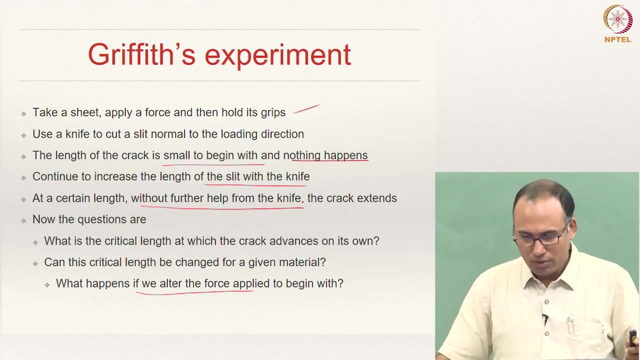 This lambda is a constant And this is the volume of the material that will actually contribute to release of the strain energy, And that energy will be utilized for creation of the surfaces. Okay, Is that clear? So the total energy released? we are talking about elastic material. 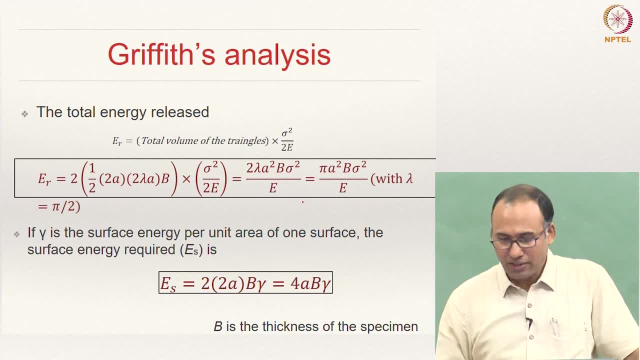 So we know linear elastic, in fact. So sigma square by 2e is your strain. energy density, is not it Per unit volume, Yes or no? All of you agree or no? Yeah, We have done that in the previous modules. 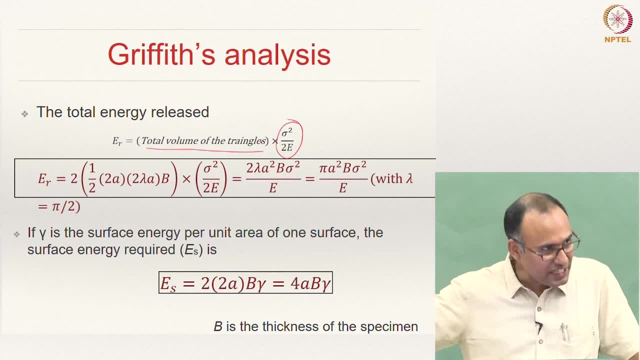 And then the volume from which this energy is being released from those two triangles. So total volume of the triangles, assuming the out of plane thickness to be capital B. Your capital B here is your out of plane thickness. So this is two triangles. 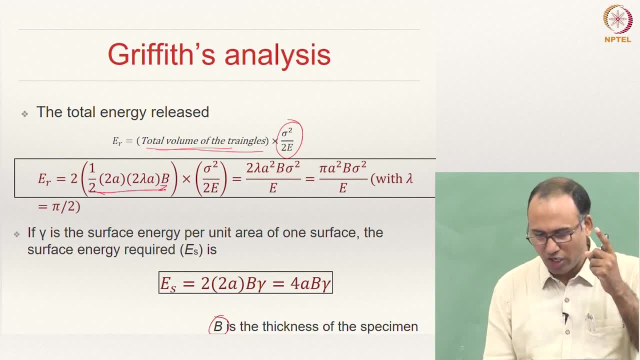 We have. this is the area of one volume, of one triangle, actually not triangle. I should not be calling it as triangle. It is a triangular, the end view is triangle, but it is extended, extruded in the direction with a, B. 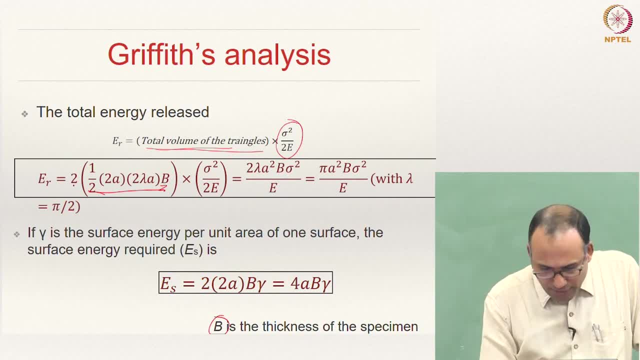 It is like a prism. So you have two of them and the volume 2 times that volume times sigma square by 2e. Okay, Okay, So this is the volume times sigma square by 2e. And now if I take my lambda equal to pi by 2, you can actually show that for lambda equal. 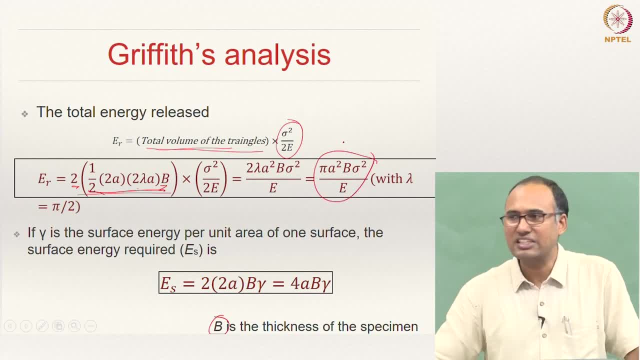 to pi by 2, this is what will be your energy release Right Now. if gamma is the surface energy per unit area of one surface, then you have how many? how many surfaces have we created? Two surfaces, So the total surface energy is 2 times 2a times B gamma. 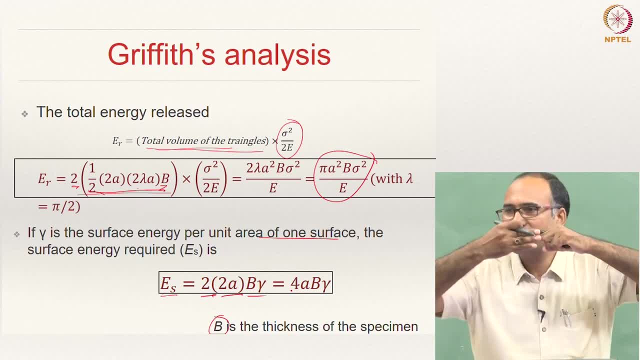 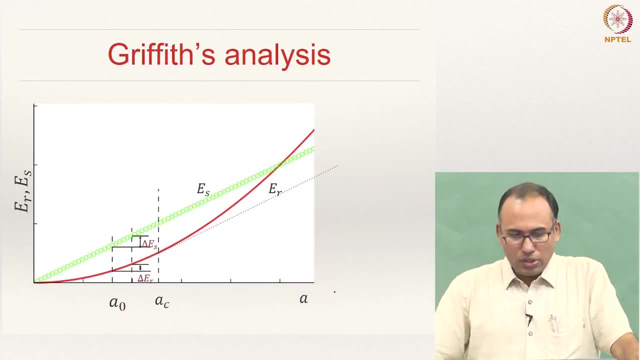 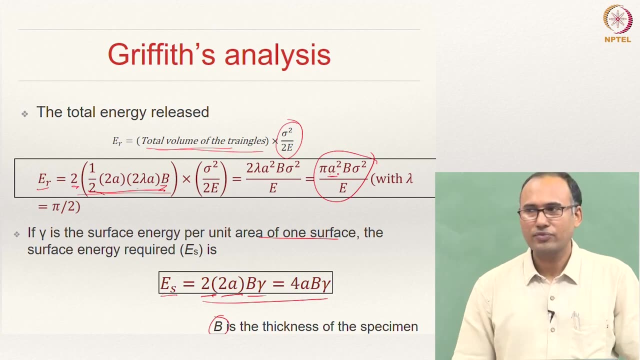 2a is this volume, 2a is this one. and out of plane thickness is B. So that is your surface energy, Right. So now, if you would plot, you can see these equations. So here released energy goes as a square. that means it is a parabola and surface energy. 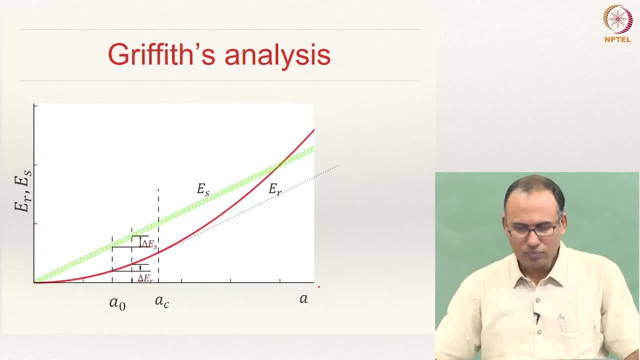 goes as a. So that means it is a straight line. Okay, So what Griffith said was When the energy release rate becomes greater than the surface energy rate. here when we say rate, it is not time rate, but it is energy released per unit crack length. 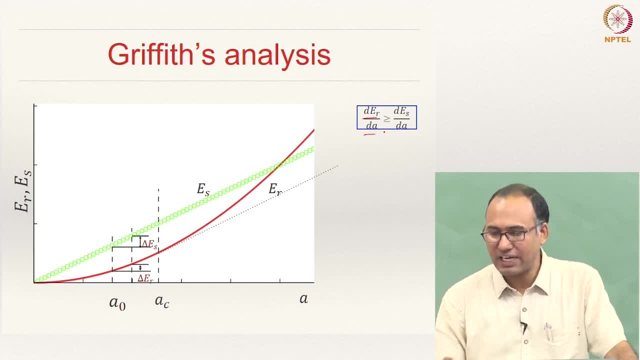 So dE, R by dA. when that becomes greater than this guy, that is when your crack properties. Okay, It should be first: energy release rate E R should be equal to E S and the rate at which E R is changing should be greater than rate at which the surface energy changes. 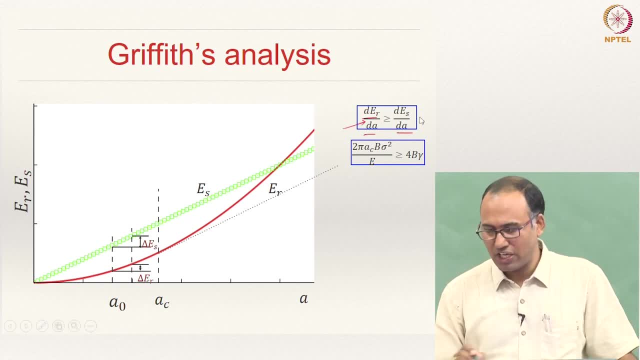 Okay, So then if you can, you know the equation for E, R and E S and you can actually show that 2 pi AC B sigma square by E should be greater than or equal to 4 B sigma gamma for crack to properties. 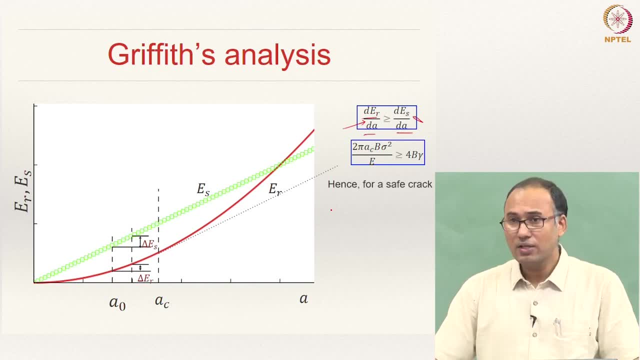 Okay. Hence, if you have to have a safe crack, you have to have a safe crack. Okay, If you have a safe crack, your critical length should be less than or equal to this number. Now the questions that we have asked: does it the critical length change from material? 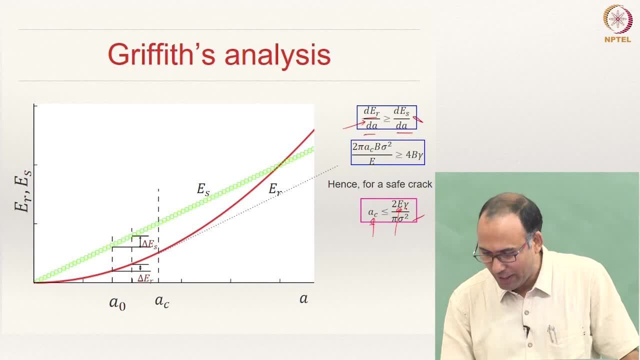 to material? Yes, it does, because it depends on the E and gamma. Does it depend on the applied force? Yes, it does, because the sigma is your applied force Right. So if you know what is my sigma, what is my initial crack length?